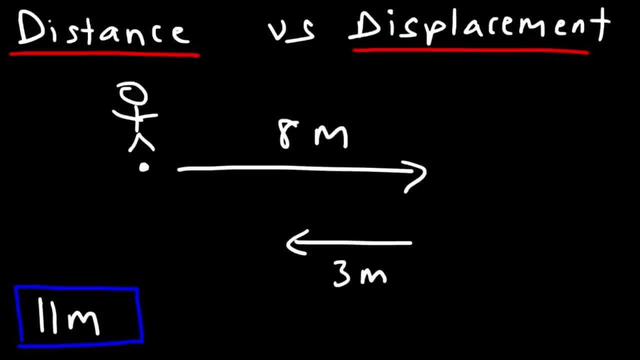 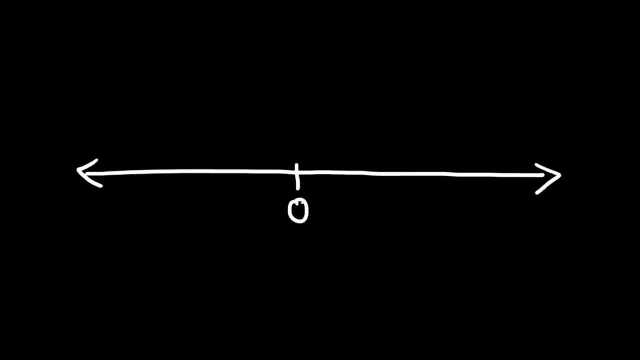 his displacement is not 11, but rather his displacement is 5 meters. Displacement is the difference between the final position and the initial position. So let's say, if we have a number line And let's say this is position 0.. So John traveled 8. 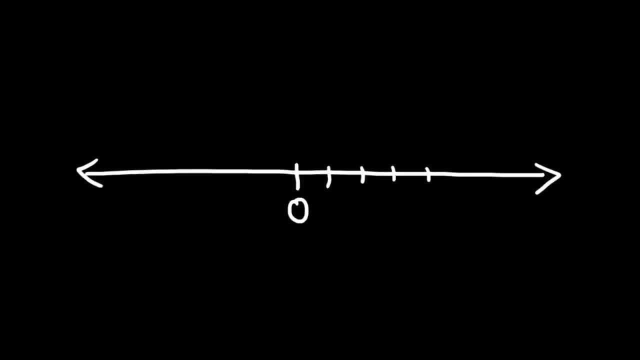 meters east. So now he's at position 8 on a number line. So during the final position, the first part of his trip, his displacement was positive 8. Then he traveled 3 meters west, So his displacement is negative 3. So now he's at position 5. And so his net displacement. 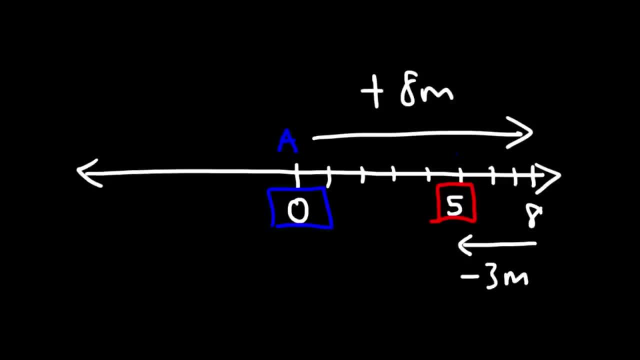 is 5 meters, because he started from position A and now he's at position B, which is located at position 5.. And so your net displacement is basically it's the final position, let's say PF minus the initial position. His final position is position 5.. His initial position is 0. So 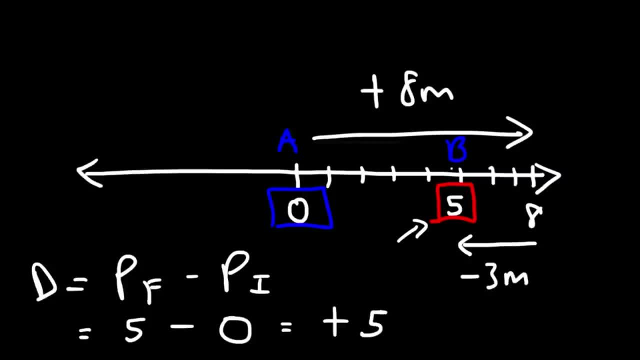 his displacement is positive: 5. He went from A to B, And so that's the basic idea behind displacement. The total distance is 11.. Now, distance is a scalar quantity. It only has magnitude. Displacement is a vector quantity. It has both magnitude and direction. 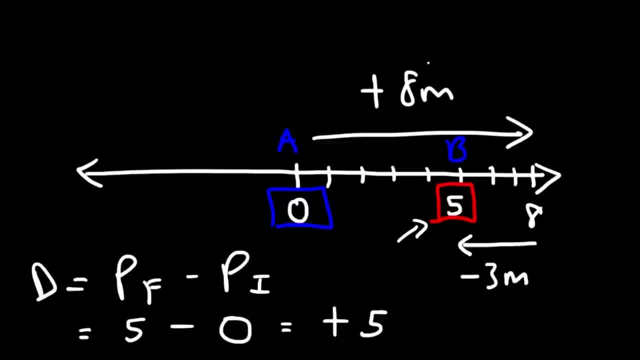 In the case of distance, in the first part of the trip he traveled a distance of positive 8.. In the second part, he traveled a distance of positive 3. And so the total distance is 11 meters. Now, displacement has magnitude and direction. 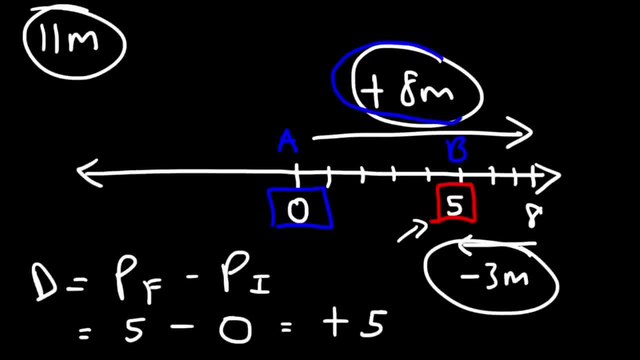 During the first part of his trip, his displacement was positive 8.. The magnitude is how far he traveled, which is 8 meters. The direction is he's traveling east, And so we have a positive sign for going in an eastward direction. Anytime you go towards the right, you're going in the 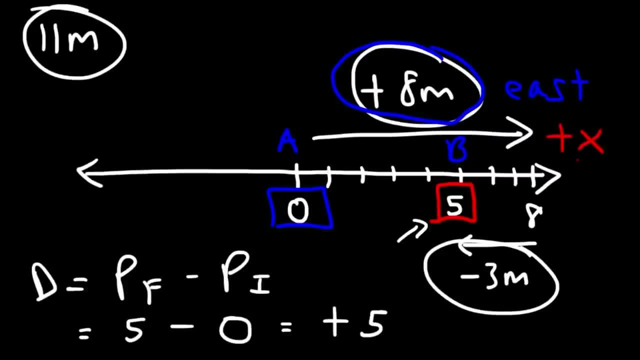 positive x direction, So the displacement is positive. Now, during the second part of the trip, he's traveling west, That is, towards the negative x direction, And so it's negative 3 in terms of displacement, but in terms of distance it's positive 3.. Keep this in mind. Distance is always positive. 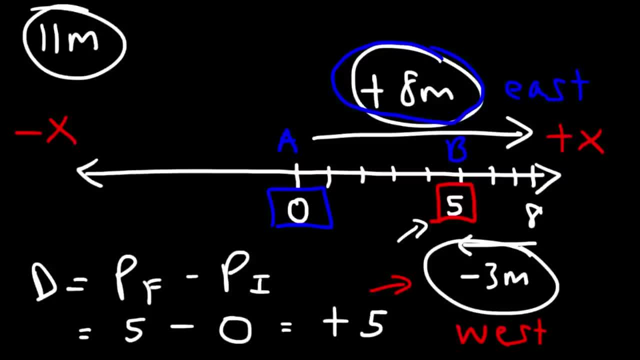 but displacement can be positive or negative. If you're traveling east or north, displacement has a positive value. If you're traveling west or south, displacement has a negative value. And so if you add up the displacement for the first part of the trip plus the displacement 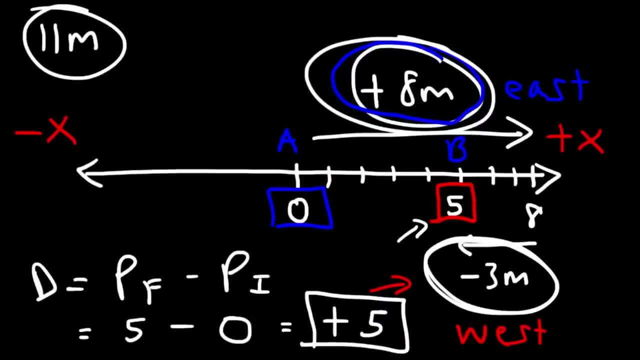 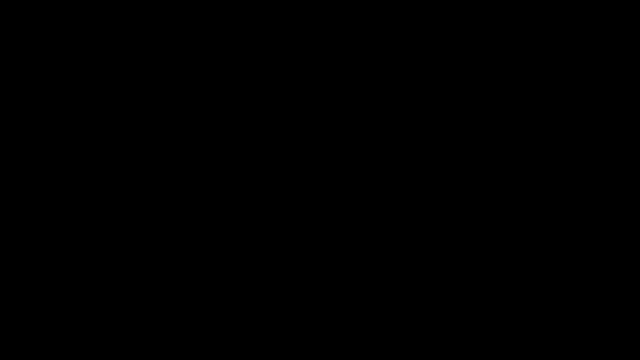 of the second part, you get the net displacement of positive 5. Positive 8 plus negative 3 will give you positive 5.. Now let's say a car travels 200 miles. Would this description be related to distance or displacement? 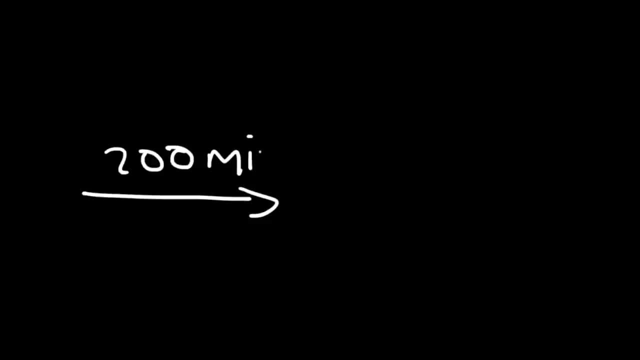 So if I say you traveled 200 miles, am I describing distance or displacement? Well, this would be a description of distance, because no direction was indicated, So you could be going east, west, north or south. If you simply state 200 miles, you're. 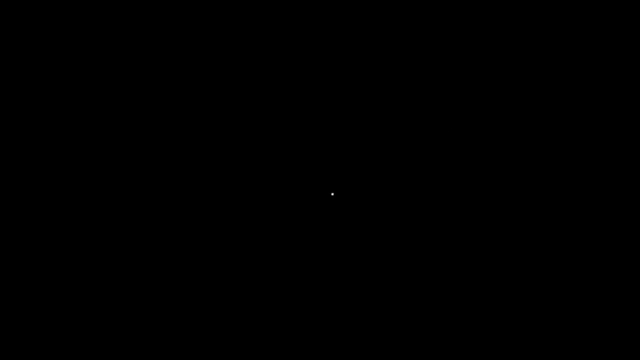 describing distance. Now, let's say if the car traveled 300 miles north, In this case I have the magnitude, which is 300 miles, and I also have the direction, which is in a norther direction. So in this case I'm describing displacement. Displacement is 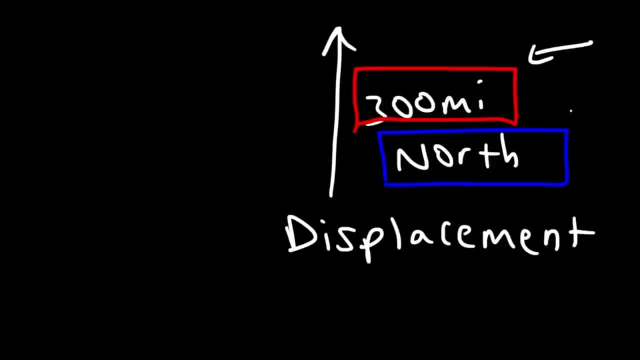 a vector quantity, It has both magnitude and direction, Whereas distance is a scalar quantity. it only has magnitude, such as 200 miles, without any direction. So make sure you understand the difference between a scalar quantity and a vector quantity, If you're. 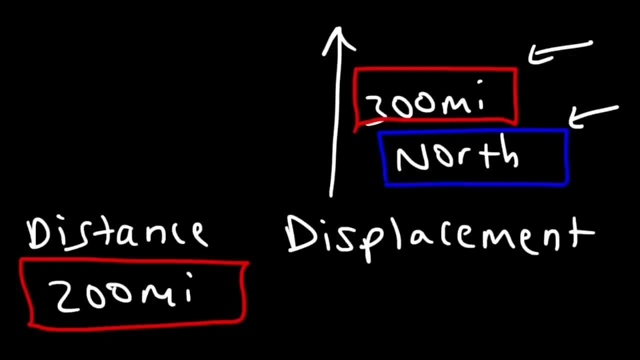 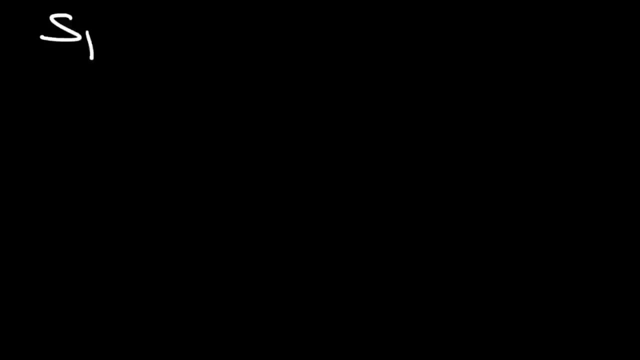 talking about distance, you're not going to be able to know the difference between a scalar quantity and a vector quantity. A scalar quantity, as we said before, has magnitude only, but a vector quantity has a magnitude and direction. Now let's talk about speed. When you think of the word speed, what do you think of Speed? 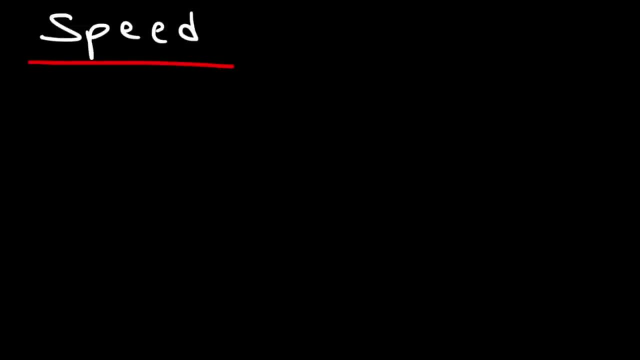 tells you how fast something is moving. So let's say, if a car is traveling 30 miles meters per second, What does that mean? So that means that every second the car will have traveled a distance of 30 meters. So let's say: this is the starting line and I'm going to use a box to 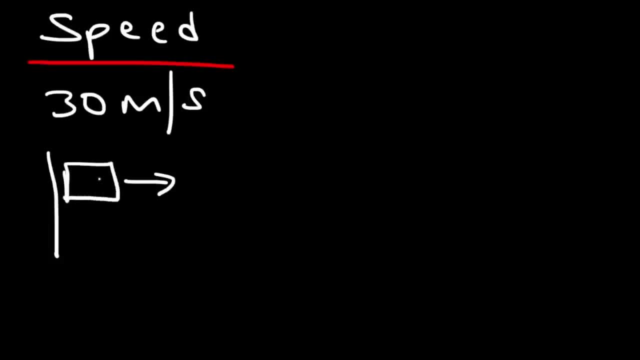 represent a car, and the car is moving in this direction with a speed of 30 meters per second. So one second later, the car will have traveled a total distance of 30 meters. Two seconds later, it's going to travel another distance of 30 meters. So for a total distance of 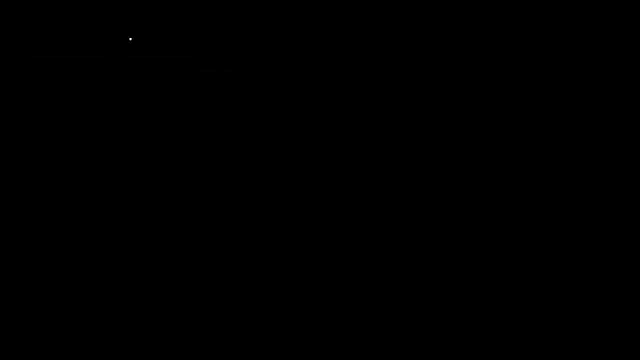 60 meters So we can make a table. So let's put t for time, d for distance. So if the speed is 30 meters per second, so every second the distance traveled will increase by 30.. And so that's what speed tells us. It tells us how fast the distance of an object or the distance 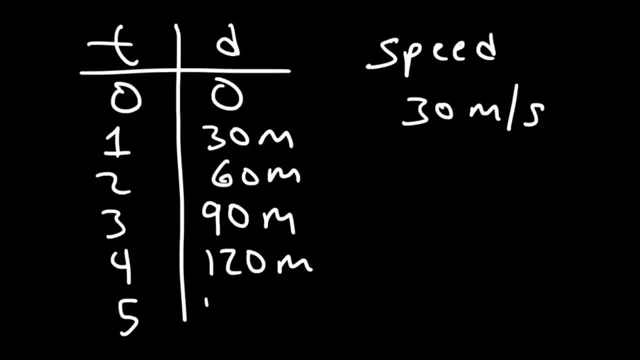 traveled by an object is changing every second. So let's say: if you're driving a car and you're going 60 miles per hour, Every hour, at that speed, you will travel a distance of 60 miles. So let's say: if you want to travel a distance of 300 miles, It's going to take you five hours to do. 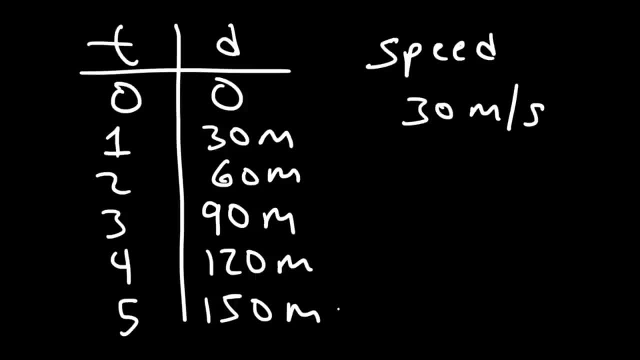 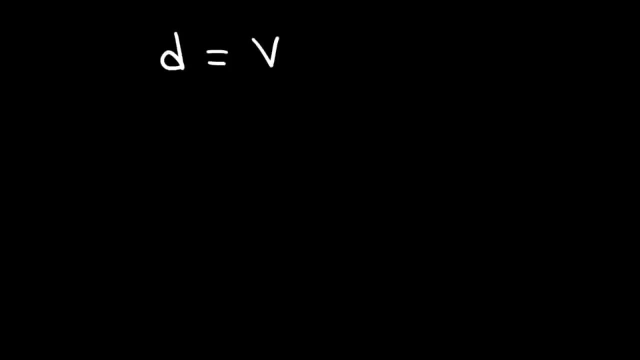 so In the first hour you're going to travel 60 miles. In the second hour you have covered a distance of 120 miles. So every hour you're going to travel an additional distance of 60 miles. Now there's a formula that you need to know, and it's: d is equal to vt. 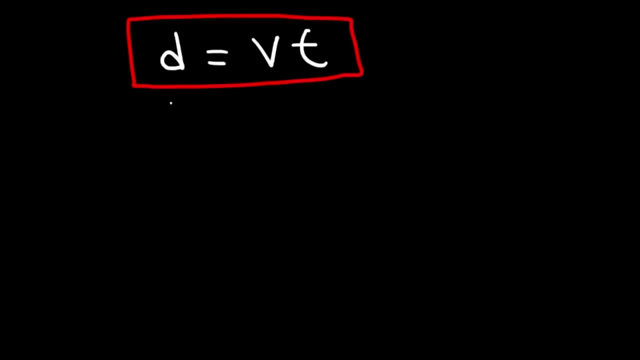 In this equation, d can be used as a distance and v represents speed, t represents time. Now, sometimes, with this formula, you could use the velocity in terms of v, And if you do so, then d will no longer technically be represented by distance, but it's going to be represented by displacement, And so 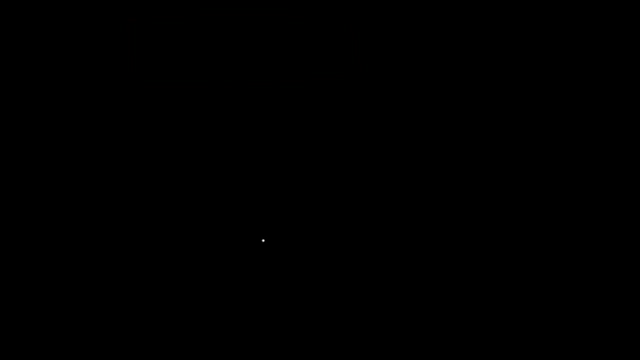 you could use that simple formula in many different ways, So here's a question for you. So let's say, if you have an object that is moving at a speed of, let's say, 50 meters per second, how long will it take for this? 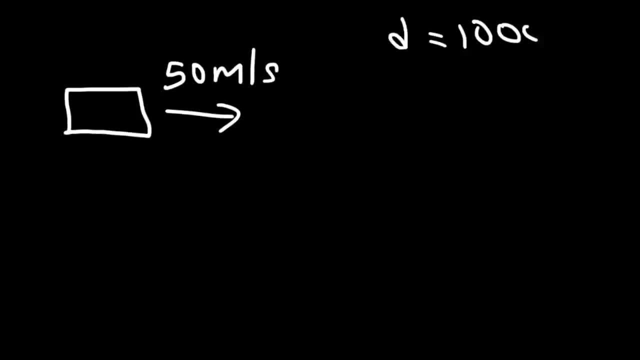 object to travel a distance of 1,000 meters, so we're looking for the time, how long, so we could use this formula: D is equal to V- T, so the distance is a thousand meters, V is 50 meters per second and we need to calculate the 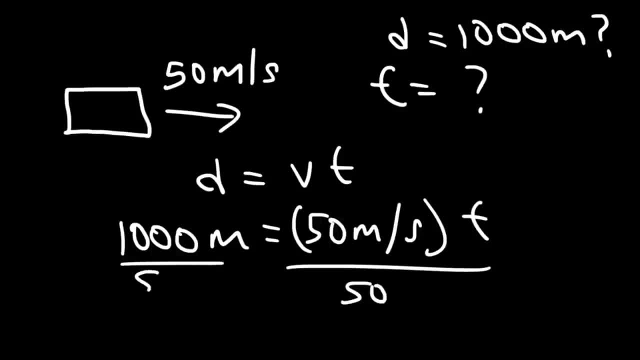 time. so we can divide both sides by 50, and so it's going to be a thousand divided by 50. if we cancel a zero, that's a hundred divided by five, which is 20. so it's going to take 20 seconds for this object to travel a distance of a. 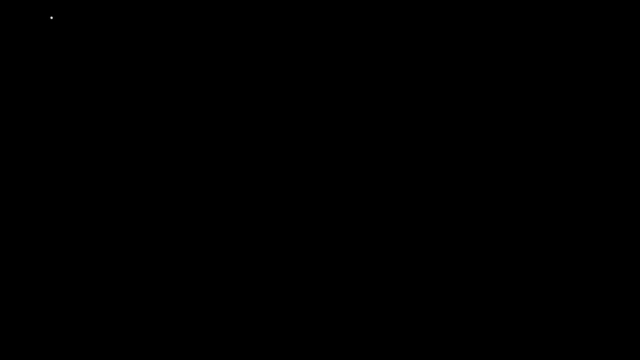 thousand meters. now let's talk about speed and velocity. so what is the difference between these two quantities? because they both describe how fast something is moving, but there's a difference between them. speed is a scalar quantity and velocity is a vector quantity. speed is always positive. velocity can be positive or negative. 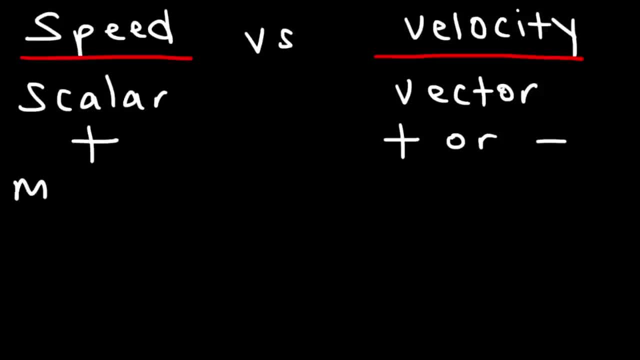 Now recall that a scalar quantity only has magnitude, whereas a vector quantity has magnitude and direction. So can you think of some examples that will distinguish speed from velocity? So let's say, if a train- I'm going to use a box again- is moving at 45 meters per second, 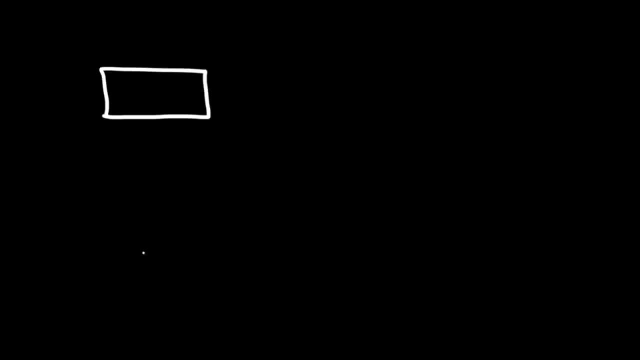 Let me take away the arrow, So you don't have any direction. It's simply moving at 45 meters per second. In this case, this describes the speed of the train, because I'm telling you how fast it's moving, but not where it's going. 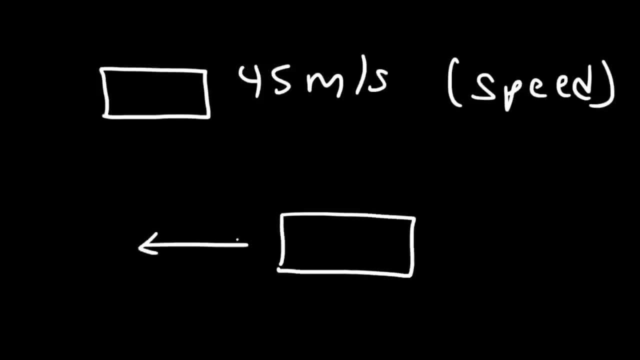 Now, let's say, if we have a train moving at 30 meters per second, going west, In this case, this is a description of velocity, Because not only do you have the magnitude of the vector, which is the speed, but you also have the direction. 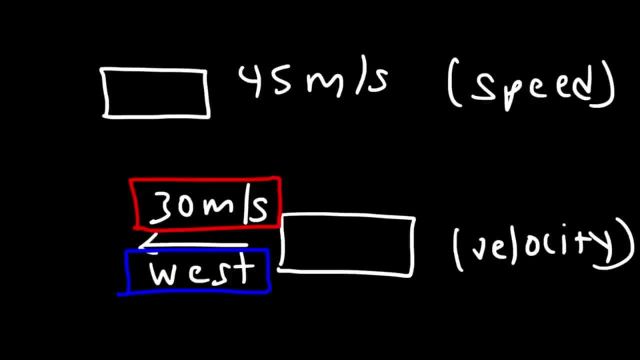 And so when you combine magnitude and direction, you have a vector quantity, And so velocity is basically speed with direction. The 30 meters per second tells you the speed, West tells you the direction, And when you combine these two you have velocity. 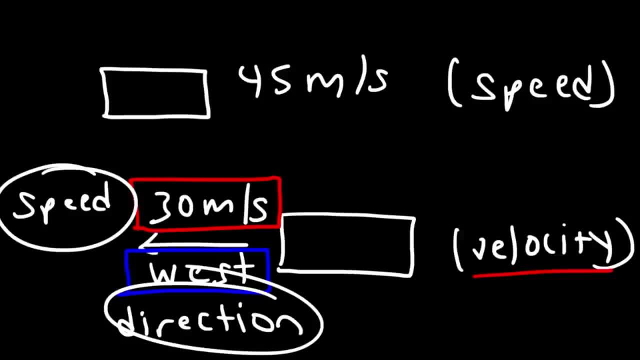 So let's summarize a few key points. Speed tells you how fast something is moving. Velocity tells you not only how fast something is moving, but also where it is going. So remember, velocity is speed with direction. Speed can only be positive. 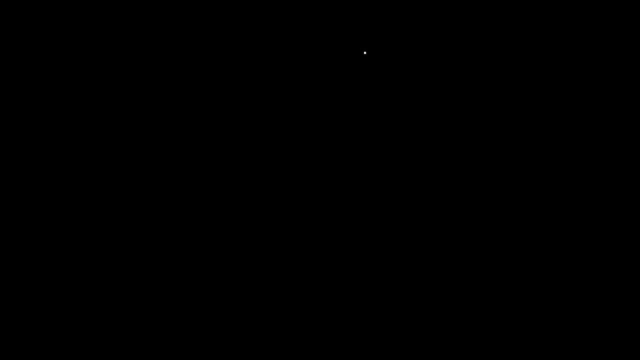 Velocity can be positive or negative. So let's summarize a few key points. So if V is negative- 20 meters per second- you know you're dealing with velocity because it's negative. If you're looking for the speed, the speed would be positive: 20 meters per second. 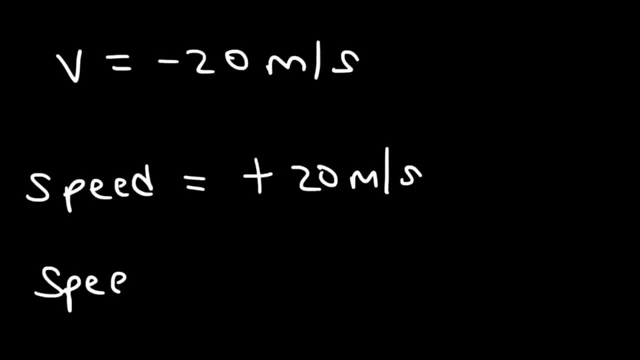 Speed is always positive And you could say that speed is the absolute value of velocity. Velocity can be positive or negative, but speed is always positive. So if the velocity was negative 35 meters per second, the speed is automatically positive: 35 meters per second. 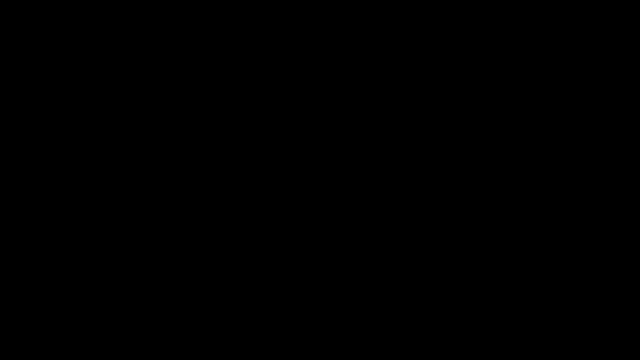 Now there are some mathematical formulas that you want to know when dealing with speed and velocity. There's something called average speed, Because sometimes in physics you need to calculate the average speed of an object. The average speed can be calculated by taking the average speed of an object. 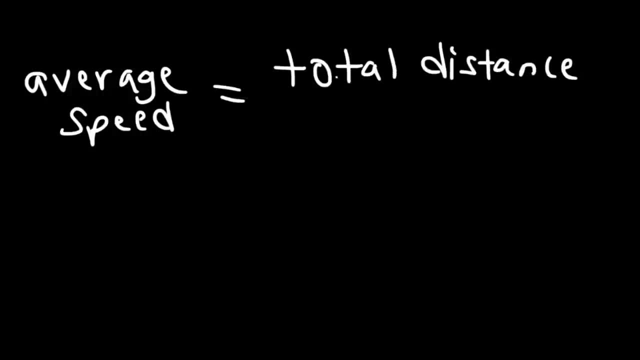 Taking the total distance traveled by the object and dividing it by the total time. Now, if you think about this, formula d is equal to vt. v can be described as the speed or the velocity. So if you divide both sides by t, you could cancel this on the right side. 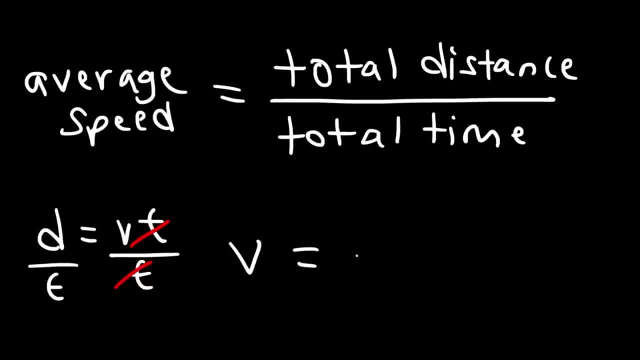 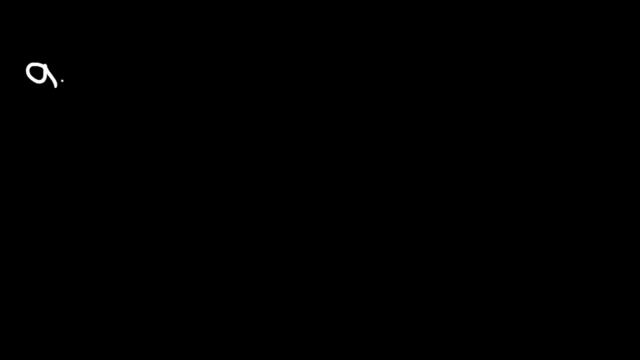 You'll see that v, which is the average speed in this case, is equal to d over t. So average speed v is equal to the total distance, d divided by the total time, t. Now what about average velocity? Let's say, if we wish to calculate average velocity, how can we do so? 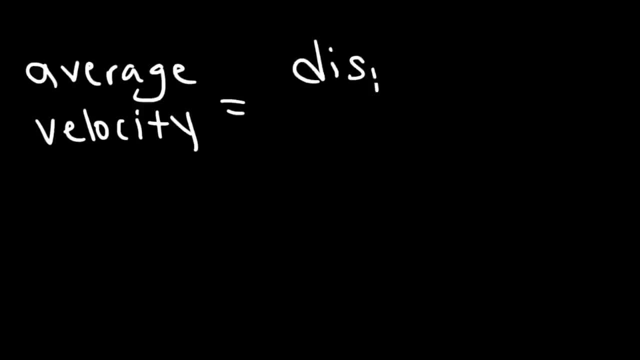 Average velocity is equal to displacement divided by the total time. So in this case we're going to calculate the average speed of an object. In this case the formula looks the same: Average velocity can be represented by v. displacement can be represented by d and. 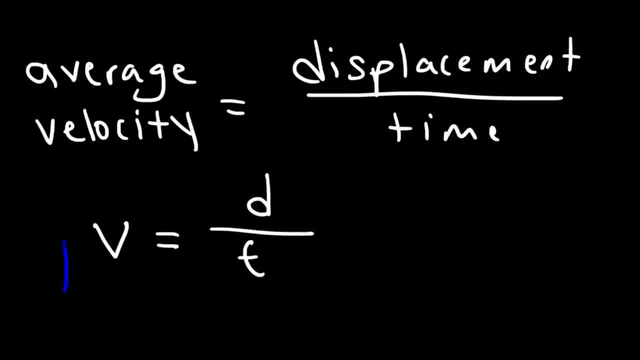 the time is t, So the formula looks identical, but the meaning is different. So keep this in mind. velocity is associated with displacement, speed is associated with distance. Now let's say, if you have an object, and this object traveled 12 meters east, and then it. 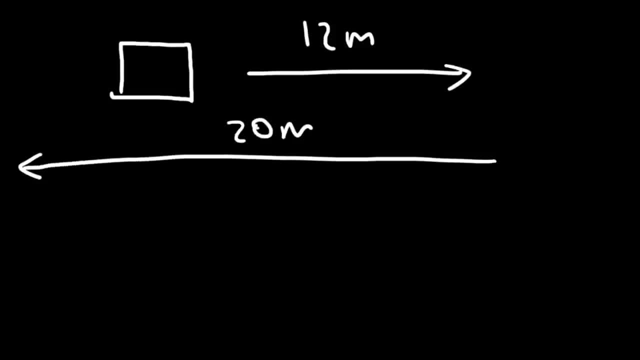 travels 20 meters west And it did so in a time period, a total time period of 4 seconds. So let's say, going from position A to position B, that's a distance of 12 meters, and from position B to position B, that's 12 meters. 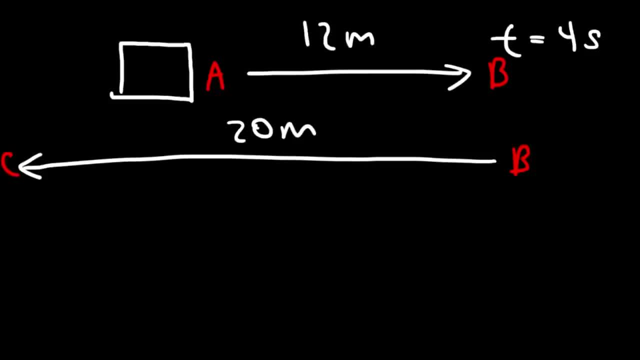 C, 20 meters, So that total trip from A to C took only four seconds. So for this object going from A to C, what is the average speed of the object And also what is the average velocity? So to calculate the average speed we need to. 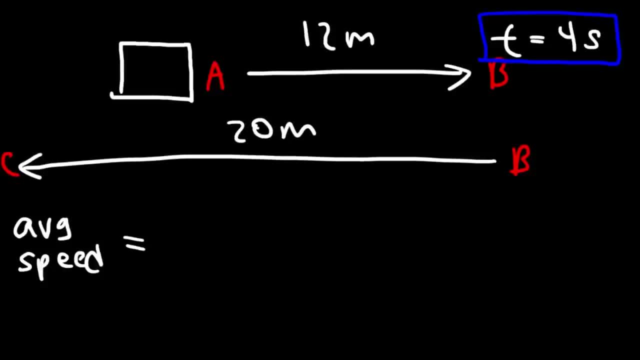 determine the total distance and divide it by the total time. The total distance is simply 12 plus 20.. If you add those two numbers, it will give you 32 meters, And the total time is 4 seconds. So 32 divided by 4 is 8.. So the average speed 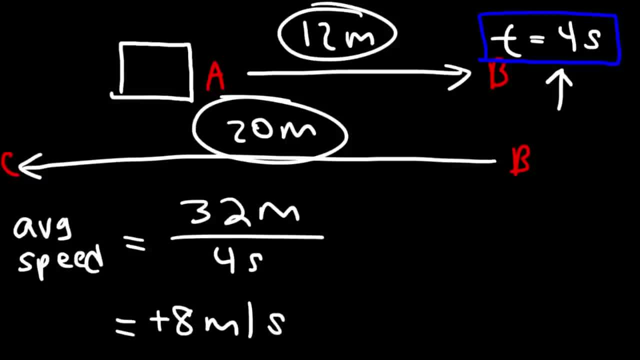 is positive 8. Keep in mind: speed is always positive. So the average speed is positive 8. Keep in mind, speed is always positive. Now, what about the average velocity? Well, we know that average velocity is defined as displacement divided by the total time. The displacement for the 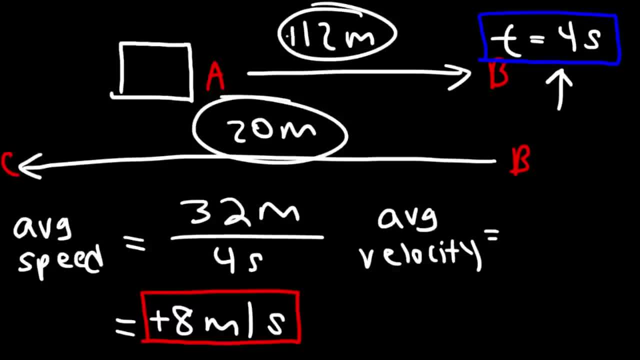 first part of the trip, going from A to B, is positive. 12, because the object is traveling in a positive X direction, The object is going east. For the second part of the trip, the object is traveling west towards the negative X direction, And so going from. 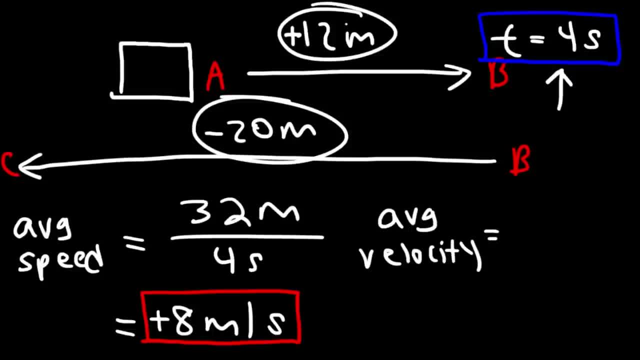 B to C, the displacement is negative. So if we add up 12 and negative 20, we can get the net displacement, which is negative 8.. Now keep in mind you can also treat this as a number line. Let's say A is at position 0.. B will be at position 12.. And then, if you do 12,, 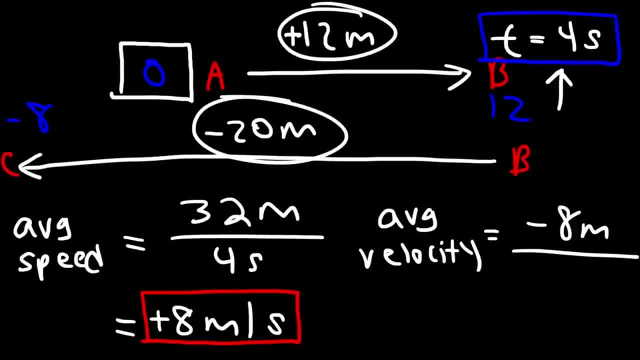 minus 20,, you'll see that C is at position negative 8. And the difference between these two positions will be the net displacement, which is still negative 8.. So the final position minus the initial position will give you the net displacement. Now let's divide it by 4. 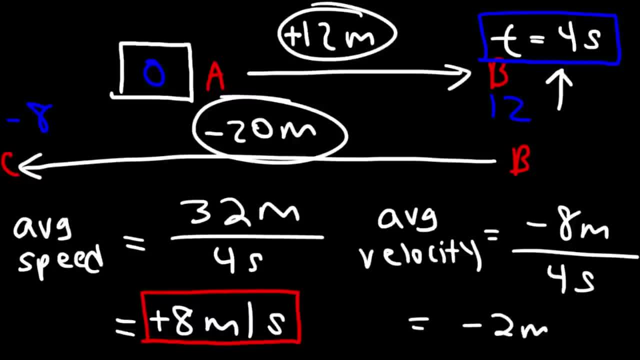 seconds, So the average velocity is negative 2 meters per second. And it makes sense because the net result is that the person traveled in the westward direction, towards the negative X axis, So going from A to C, ignoring B, the person traveled towards the west And 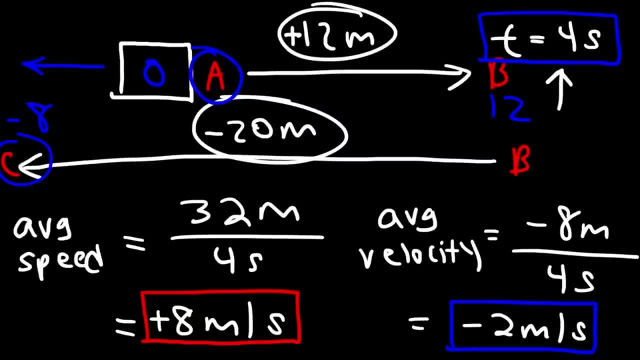 that's why the velocity is negative, because anytime you're going in the west direction, towards the negative X axis, it will be negative. If you're going towards the positive X axis or in the eastward direction, it's going to be positive. 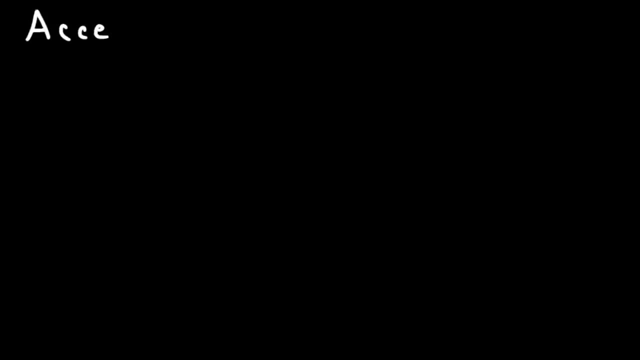 Now let's talk about acceleration. What is acceleration? Now, you've encountered acceleration when driving a car. A good way to think about it is: imagine two vehicles, let's say a truck, A car- not the most artistic person, but we'll work with this- and let's say a sports. 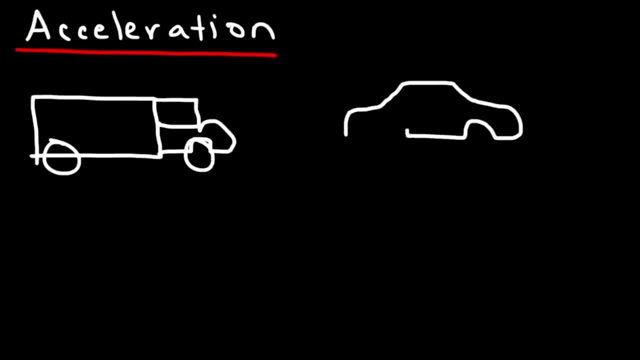 car. which of these two vehicles have, let's say, a greater acceleration? is it the truck or the sports car? so what is acceleration? acceleration tells you how fast the speed is changing or, more technically, how fast the velocity is changing. so the truck can probably go from 0 to 60 miles, and maybe let's say, 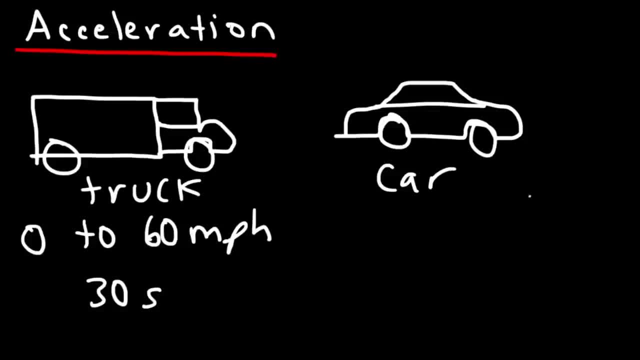 30 seconds. a sports car can go from 0 to 60 in a shorter period of time, let's say in 5 seconds. so because the sports car can get through the speed of the truck, it can go from 0 to 60 in a shorter period of time. 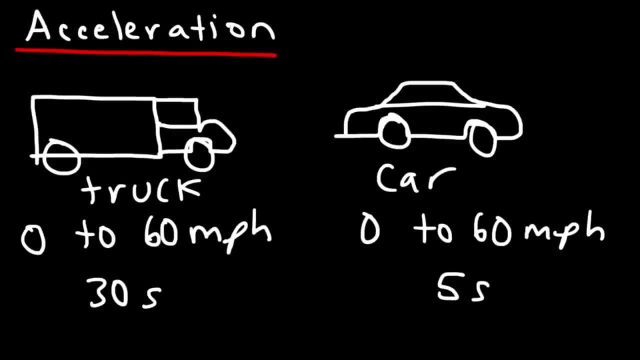 to a higher speed or to a certain speed faster than the truck, it has a greater acceleration, and so acceleration tells you how fast the velocity is changing. acceleration is defined as the change in velocity divided by the change in time, or sometimes you could just put T, so you can write it this way: 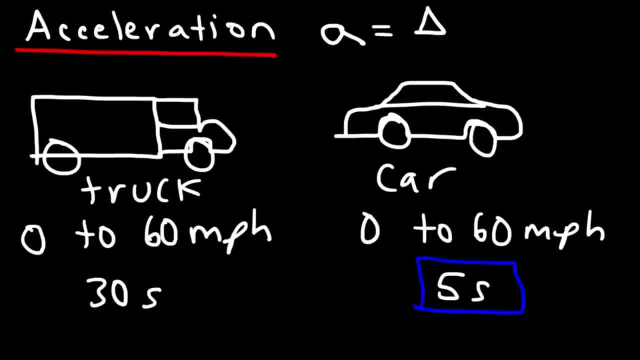 let me just the formula. so if you see the triangle, it simply makes change. so acceleration can be been this way: is the final velocity minus the initial velocity divided by the time. so to calculate the acceleration of the truck, notice that the change in the lossy is 6060I. 0 is sixty divided by the time. 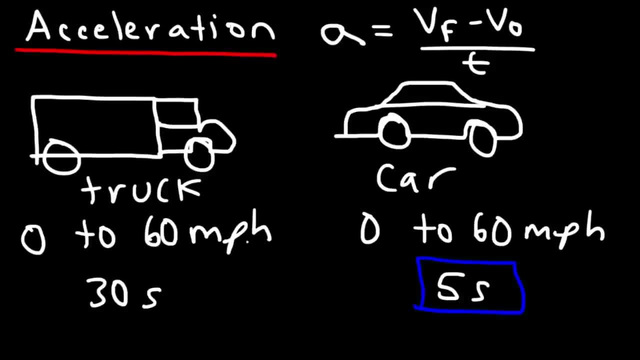 which is 30, 60 divided by 30. jus too re 80 E. this truck is two miles per hour per second because we divided miles per hour by seconds, so it's miles per hour per second. now. the acceleration of the sports car is 60 miles per hour. that's the change in velocity divided by five. 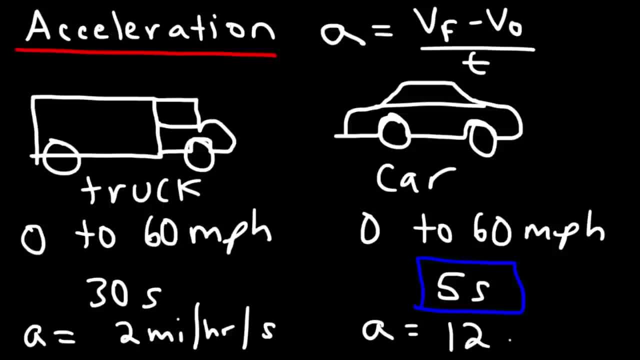 seconds. 60 divided by five is 12, so it's 12 miles per hour per second. as you can see, the acceleration of the sports car is much greater than the acceleration of the truck. the truck is going to take a long time to go from 0 to 60, but the 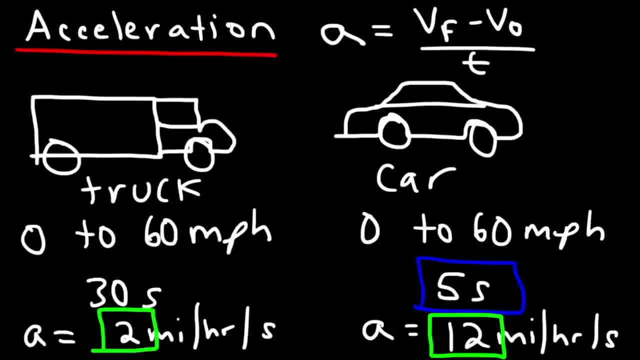 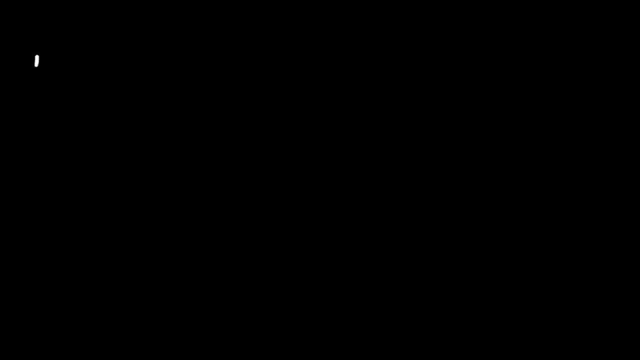 sports car will get there a lot faster, and so it has a greater acceleration. and so that's the basic idea behind acceleration: it tells you how fast the velocity is changing. now let's make a table. let's say, if an object is moving with an initial speed of 12. 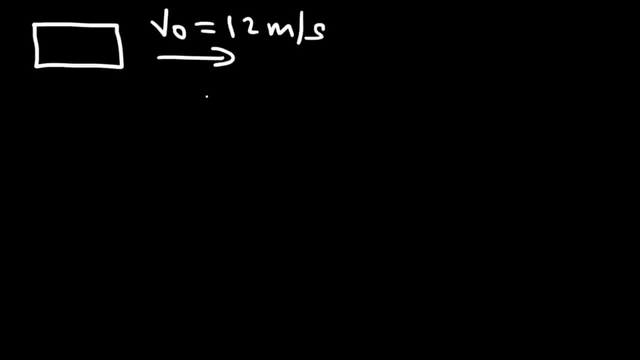 meters per second. so vo tells you initial speed or initial velocity. now, since I have an arrow, let's say it's going east. this now is: it becomes the description of velocity if I put direction with it. let's say, at this point this object or vehicle begins. 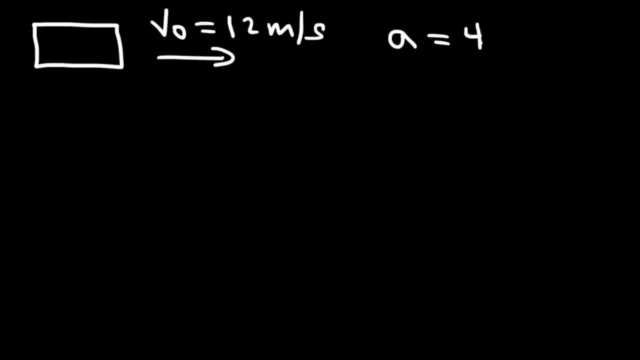 to accelerate at a rate of four meters per second squared. so this is four meters per second, per second. so what does that mean? so if we make a table, if we plot time and velocity, let's say the final velocity at a certain time at t equals zero. 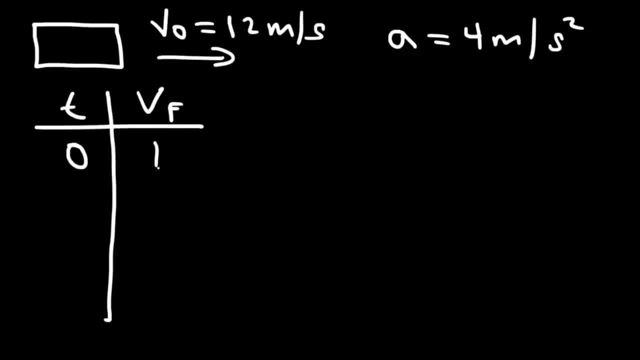 this becomes the initial velocity, so it's 12. what would the velocity be one second later? well, the acceleration tells us how fast the velocity is changing. so because the acceleration is positive, for that means that the velocity is increasing by four meters per second, every second. so anytime acceleration is positive. the 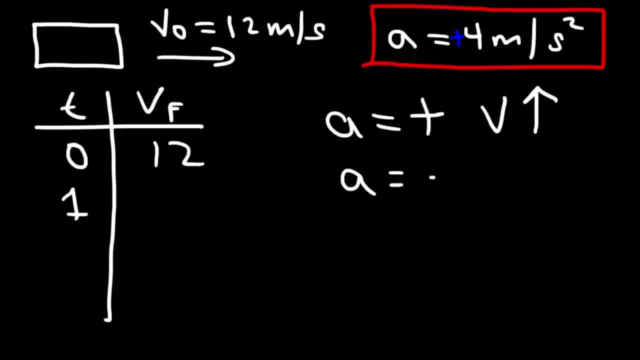 velocity is increasing. anytime the acceleration is negative, the velocity is decreasing. so one second later, the velocity will now be 16, two seconds later the velocity is 23, seconds later it's 24, four seconds later it's 28, and so every second the velocity will. 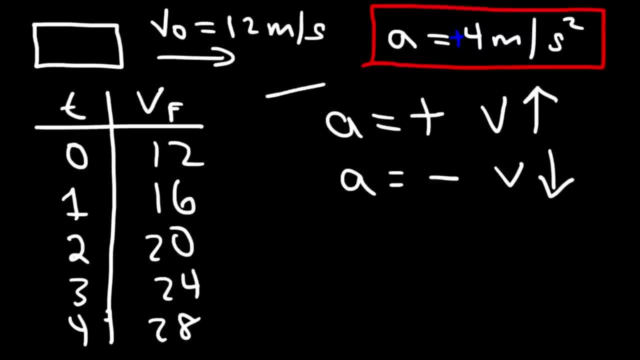 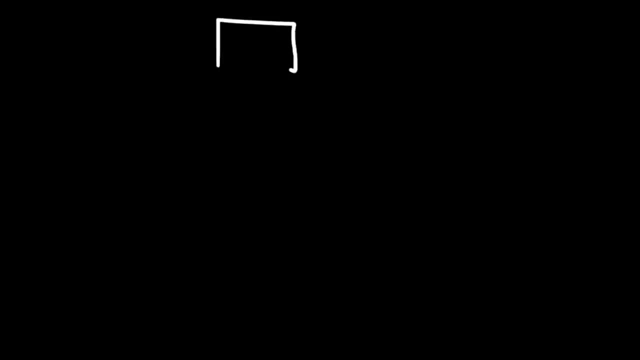 increase by four meters per second because the acceleration is four meters per second, per second. now the formula that you want to use to calculate final velocity is this equation: the final is equal to the initial plus 80. now let's say we have another object that is moving in an eastward direction at a speed of let's. 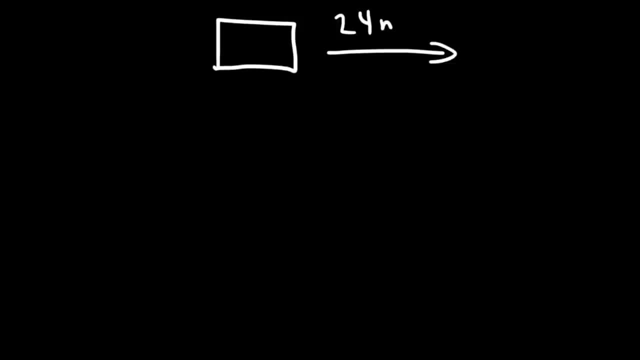 say 24 meters per second, but this time let's say the acceleration is negative, six meters per second squared. what's going on here? is this object speeding up or slowing down whenever the acceleration and velocity whenever they have opposite signs? the object is slowing down whenever they have the same sign. it's. 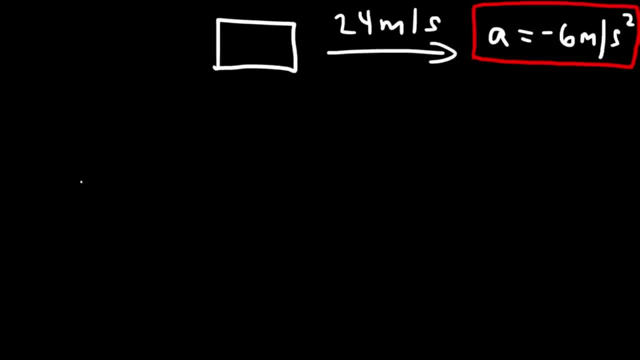 speeding up. in the last example, the acceleration was positive for and the velocity had positive values. it started with positive 12 and so, because velocity and acceleration have the same sign, the object was speeding up. so you may want to write this down: the object will be speeding up, that is, the speed will be increasing if acceleration 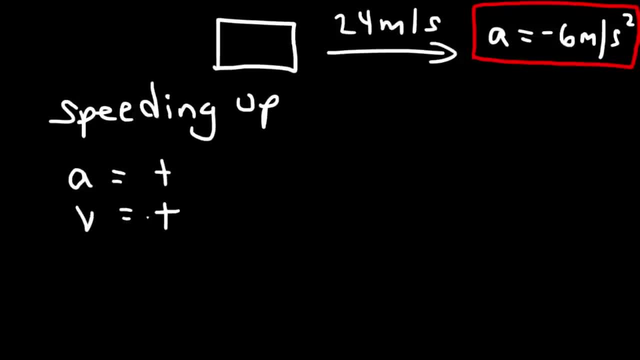 and velocity have the same signs, if they're both positive or if they're both negative. the object will be slowing down if the acceleration and velocity have opposite signs, either positive and negative, or negative and positive, and this example will illustrate that. so this time we're going to make a table. 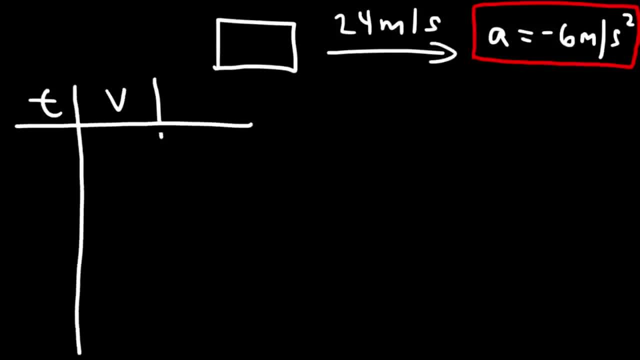 with time, velocity and velocity, and I'm going to use s for speed or SP for speed. so at t equals zero, the velocity is positive 24 and remember, speed is the absolute value of velocity. so the speed is positive 24. now, one second later, what will be the new? 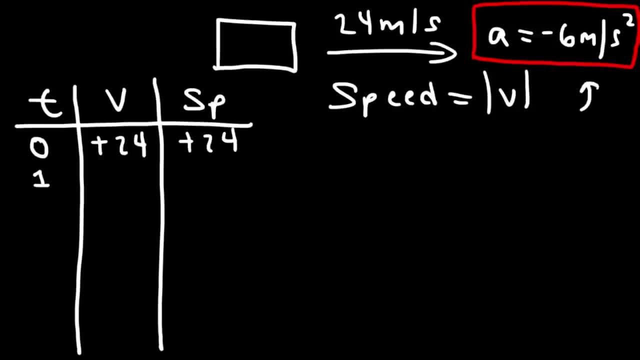 velocity. well, the acceleration is negative six, and recall that if acceleration is negative, the velocity will be decreasing. so it's going to decrease by six. so 24 minus six is 18. two seconds later it will be 12. three seconds later it's going to be six. four seconds later it's zero five. 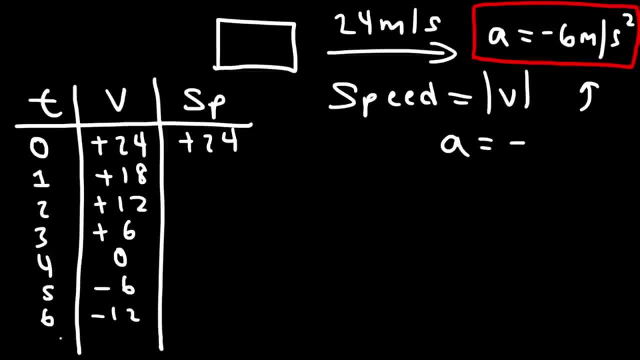 seconds later it's negative six, and then so forth. now speed is always positive. it's the absolute value of velocity. so here the speed is positive: 18 positive 12 positive 60 positive six positive 12, and so forth. now let's focus on the first half. in the first four seconds, the object is slowing. 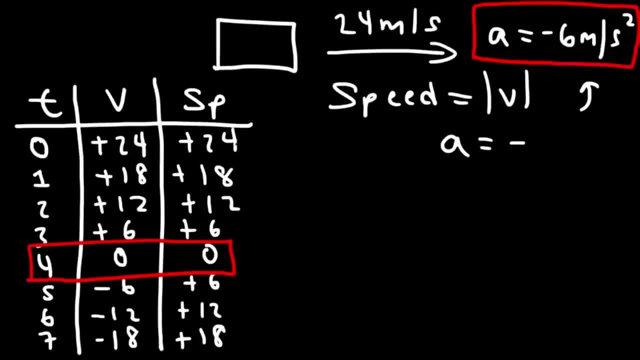 down. if you look at the speed, the speed is decreasing from 24 to zero. so what's happening is that the object is moving, But over time it's moving slower and slower and slower, And so at 4 seconds, at that instant, it's not moving. 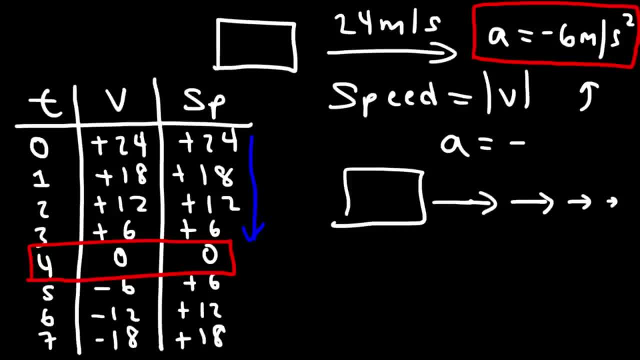 However, it's changing direction. Notice the velocity: It's going from positive to negative, Which means that it's changing from an eastward direction to a westward direction And it begins to move faster towards the west. So, as you can see, it's speeding up because the speed is increasing. after 4 seconds, 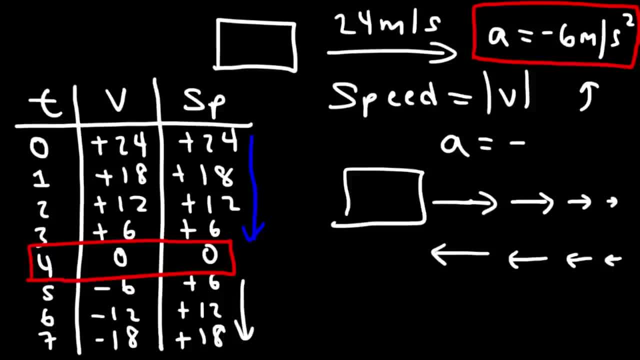 Now remember what we said before: If acceleration and velocity, if they share the same sign, then the object will be speeding up, That is, if they're both positive or both negative. But if they have opposite signs, then the object is slowing down. 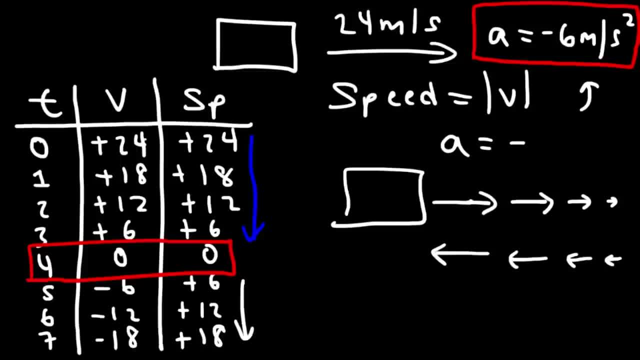 So during the first 4 seconds, The velocity is positive and the acceleration is always negative. Therefore, because the signs are opposite, it's slowing down. The speed is decreasing from 24 to 0.. Now, during the second part of this problem, that is, after 4 seconds, 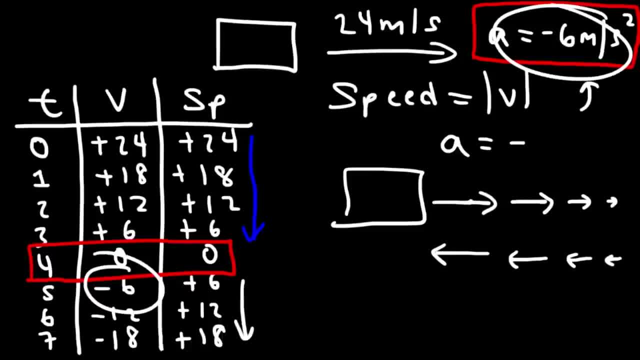 The velocity is negative and the acceleration is negative. So, because they share the same sign, The object is slowing down. The speed is decreasing from 24 to 0.. The object is speeding up. As you can see, the speed increases from 0 to positive 18 in the next 3 seconds. 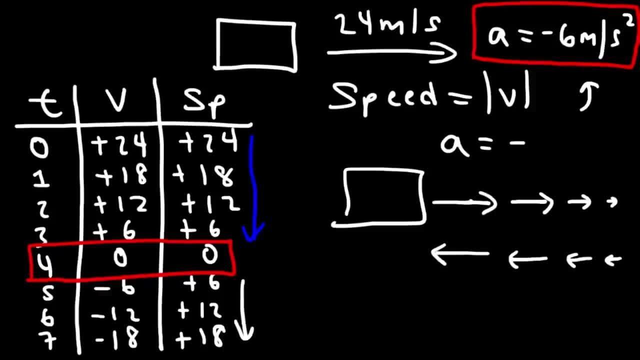 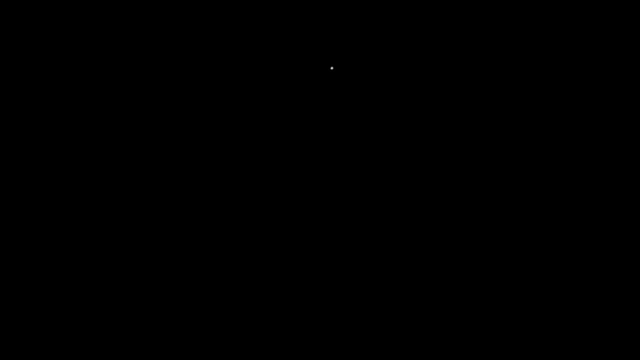 So make sure you understand that concept. If acceleration and velocity share the same sign, the object is speeding up. If they have opposite signs, it's slowing down. Now let's move on to gravitational acceleration. In physics, you'll see this symbol that looks like a G. 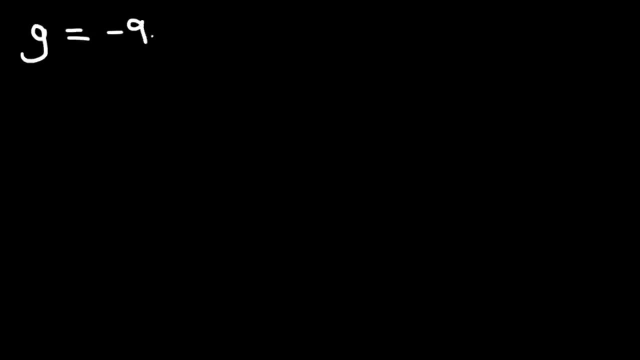 And it's equal to negative 9.8 meters per second squared. So this is the gravitational acceleration of planet Earth And it varies for different planets and other very large objects. So the gravitational acceleration of the moon, for example, is negative 1.6 meters per second squared. 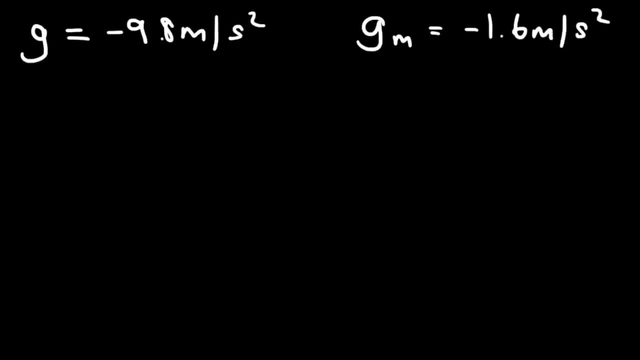 It's a lot less For one reason: the moon has less mass, Less mass than the Earth, And so you will weigh a lot less on the moon. You'll feel lighter on the moon, And so you can jump higher on the moon. 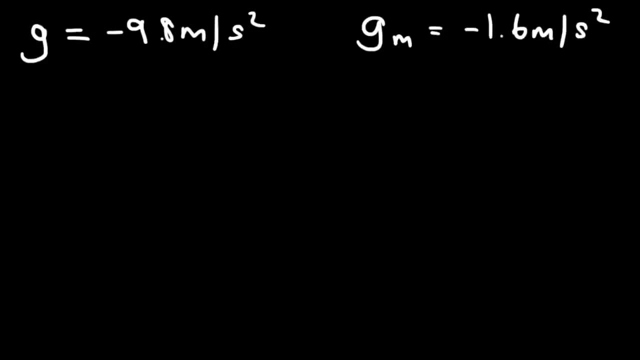 But let's focus on the gravitational acceleration of the Earth: Negative 9.8.. What does that mean? Well, in the last example we saw what a negative acceleration can do to velocity, And so the fact that this gravitational acceleration is negative means that 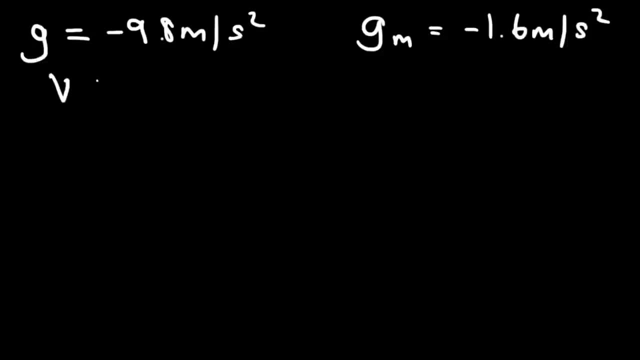 And so the fact that this gravitational acceleration is negative means that it will always decrease the velocity. Now, the gravitational acceleration of the Earth. it acts in the Y direction and not in the X direction, And so let's talk about velocity. Velocity is a vector. 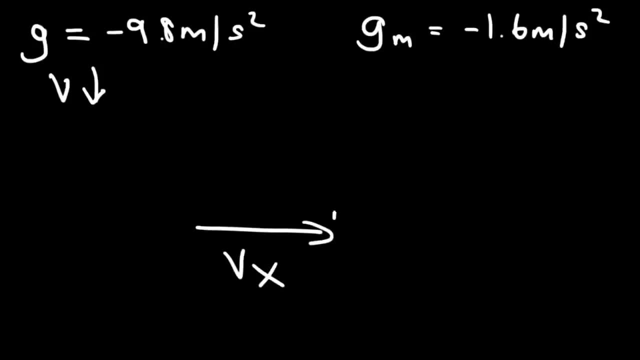 And it can have an X component and it can have a Y component, And so let's talk about velocity. Velocity is a vector. Velocity is basically the hypotenuse of this right triangle. Vx is the horizontal component of this velocity vector. 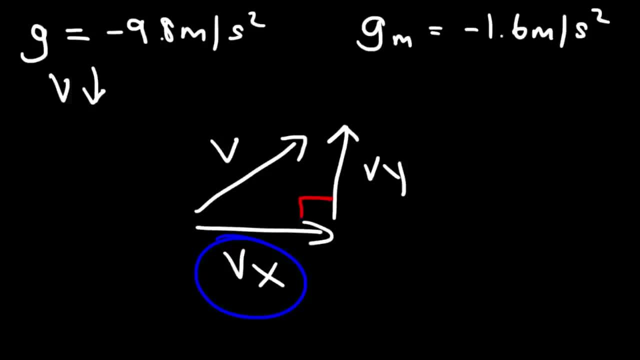 Vy is the vertical component. The gravitational acceleration does not affect Vx, It affects Vy, So technically you can write this as Gy. It's a vertical gravitational acceleration affect the horizontal velocity. it affects the vertical velocity. to make sure you understand that now let's use an example to help us understand: G- Y. 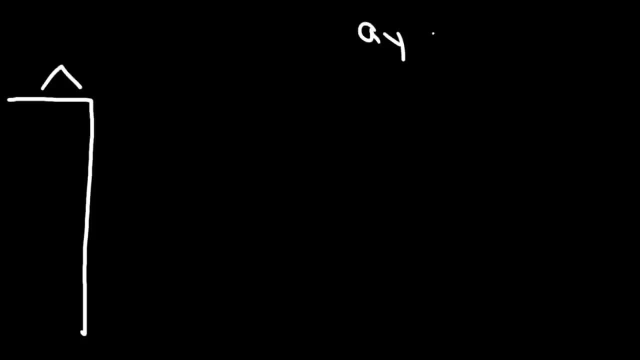 sometimes it could be written as a Y, so a Y and G are basically the same. it's negative 9.8. let's say we have a person who is standing on top of a cliff next to the ocean and this person has a ball in his hand and he released the ball. 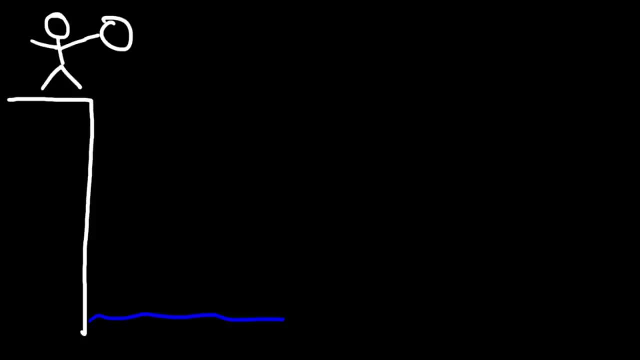 from rest, so he doesn't throw it down or throw it up, he simply let's go of the ball. well, we know what's gonna happen: gravity is gonna cause the ball to fall. now what can we do to help us understand G? Y? can you tell me about V? Y, the vertical velocity of the ball over time, will it? 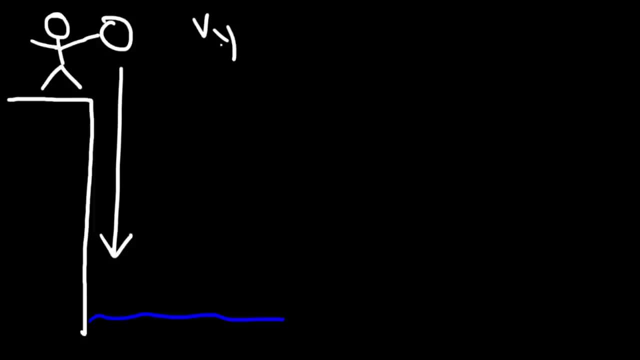 become positive or negative. we know that velocity is speed with direction, and right now the ball is going to be moving in the negative y direction. so this is positive X, this is negative X. positive Y, negative Y. it's going down you in the negative y direction. so V? Y will become negative. if we make a table with 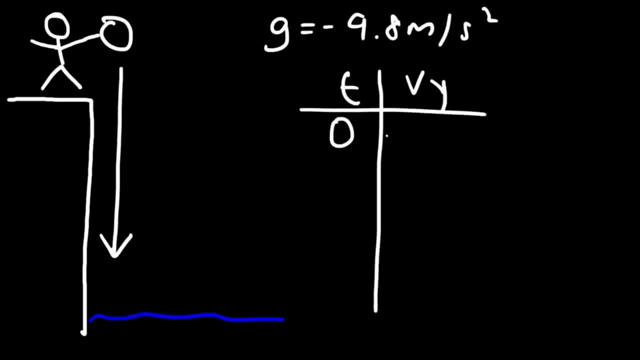 T and VY. at T equals 0, the initial vertical velocity will be 0 because the ball was released from rest. now the acceleration, or also called acceleration due to gravity, is negative: 9.8. because it's negative, the vertical velocity will be decreasing. So every second it's going to. 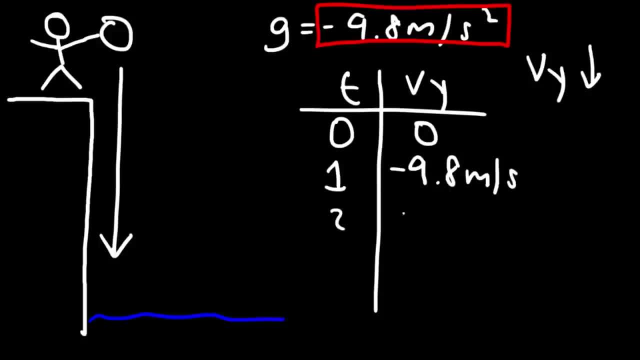 decrease by 9.8.. So 2 seconds later it's going to be negative 19.6.. 3 seconds later, it's negative 29.4.. Now the speed is always going to be positive. So if you were asked what is the speed? 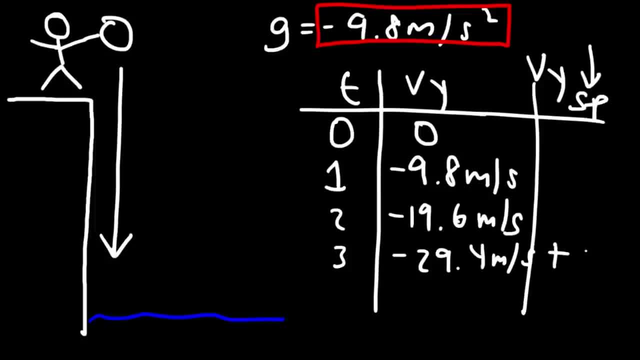 of the ball, Let's say, 3 seconds later, it's going to be positive, 29.4 meters per second. But if a test question asks you for, let's say, the velocity of the ball 3 seconds later, you should say it's negative, 29.4 meters per second, because it's going in the negative y. 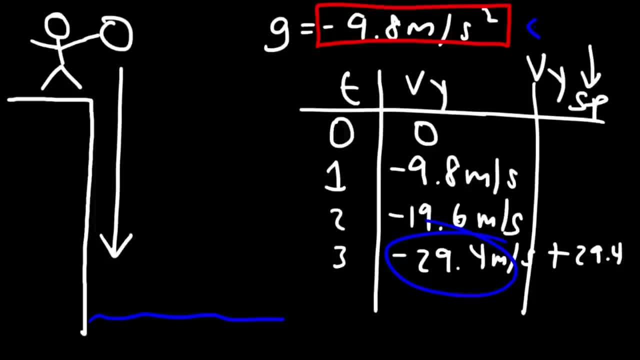 direction, And so hopefully this number makes more sense. So the gravitational acceleration tells you that the velocity of the ball is going to decrease by 9.8.. So the velocity of the ball tells you how fast the vertical velocity is changing every second. So on the moon, where g 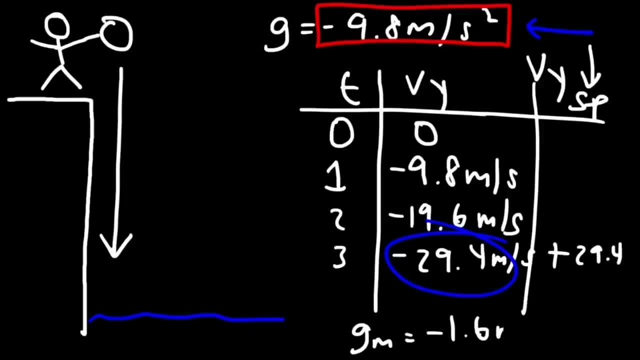 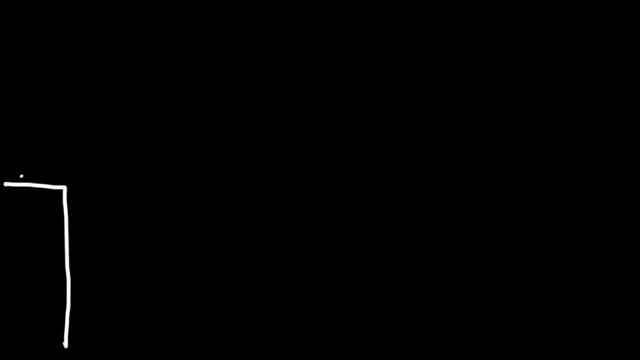 is negative 1.6,. if you were to drop a ball, the vertical velocity will decrease by 1.6 meters per second, every second. So let's say we have a similar situation. We have the same person with the ball in his hand. 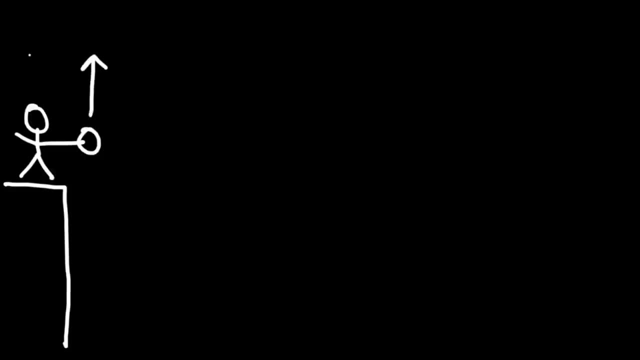 And this time he throws it in the upward direction with an initial speed of 29.4 meters per second. What can you tell me about the vertical velocity and its values every second? And let's say this person is still on the earth- where g is negative- 9.8 meters per second, squared. 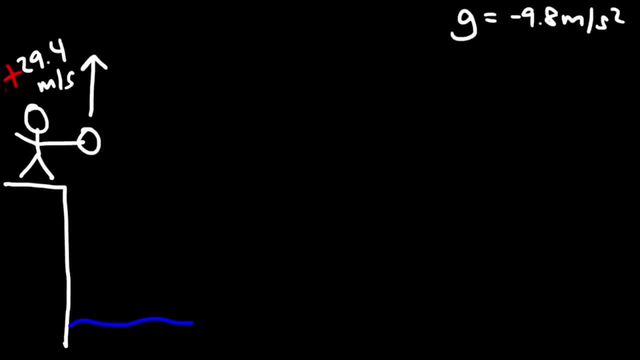 So, even though right now the velocity is positive because g is negative, the vertical velocity will decrease. So, as the ball goes upward, it's slowing down because the velocity is positive and the acceleration is negative Because they're opposite in sign. the ball is slowing down. Eventually the ball will reach. 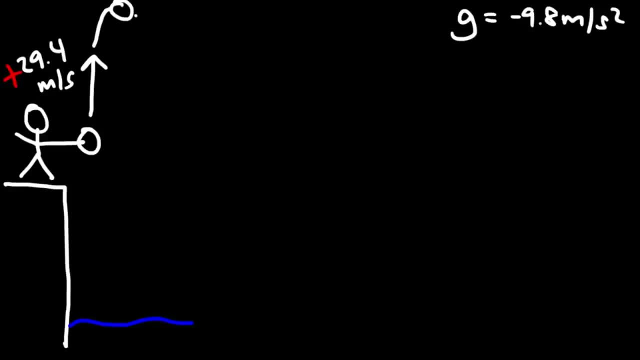 its maximum height and then it's going to change direction and begin to fall down. So if we make a table between t and vy, we're going to get the following values: So at t equals 0, that is initially the vertical velocity. 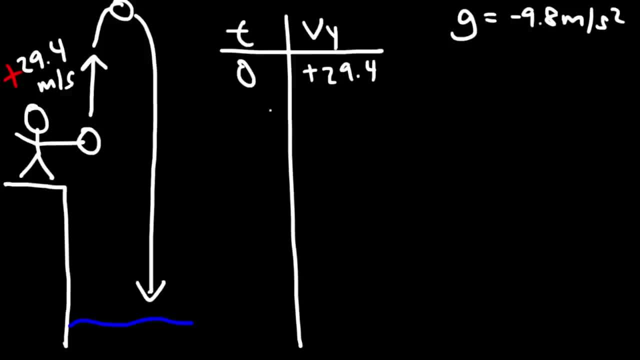 is positive, 29.4.. Now the acceleration tells us how fast or how much the velocity changes every second. So one second later it's going to decrease by 9.8.. So 29.4 minus 9.8 will give us. 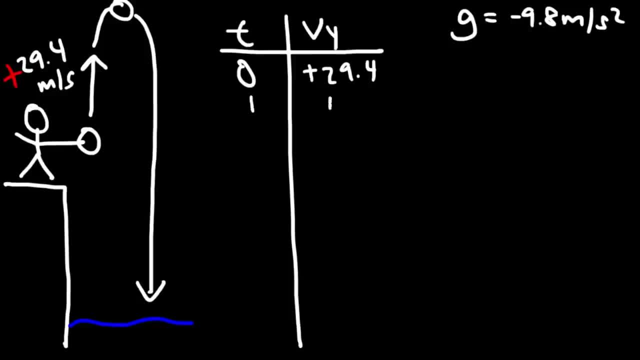 19.6.. So one second later, it's going to be positive 19.6.. Two seconds later, we need to decrease this again by 9.8.. So it's going to be positive 9.8.. Three seconds later, it's going to be at 0.. 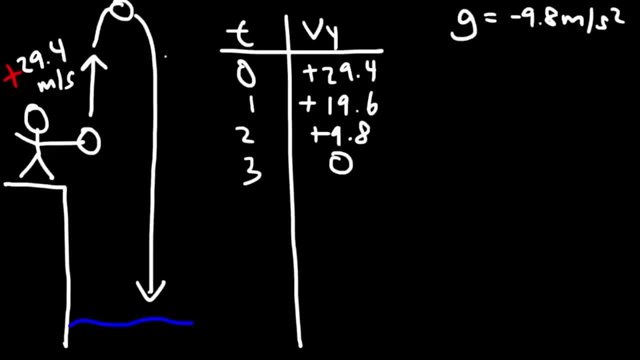 So when the vertical velocity is at 0, that means that it's no longer going up anymore and it's not going down yet It has reached its maximum height. So it took three seconds to get to its maximum height. So let's call this position A, position B and position C. So when t is 0, it's at 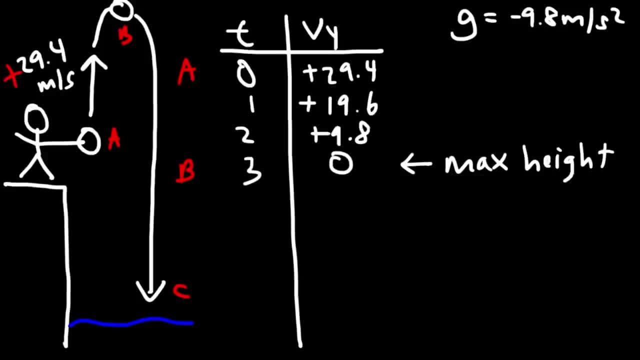 position A. When t is 3, it's at position B. Four seconds later, it's going to be negative 9.8.. Five seconds later, negative 19.6.. Six seconds later, negative 29.4, and so forth. 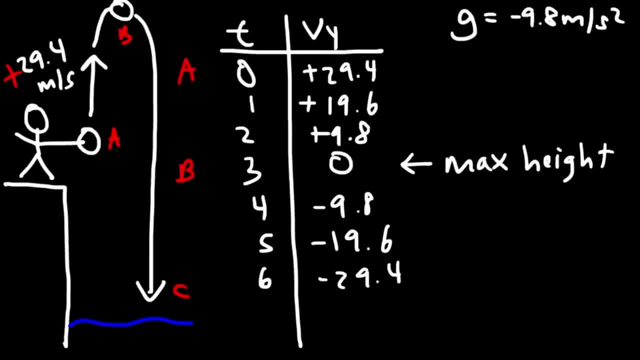 And so once it gets to position B, once it passes that position, the velocity will be negative, because it's now going in the downward direction or in the negative y direction. So that's the mathematical profile of this situation. So now you understand what's happening. 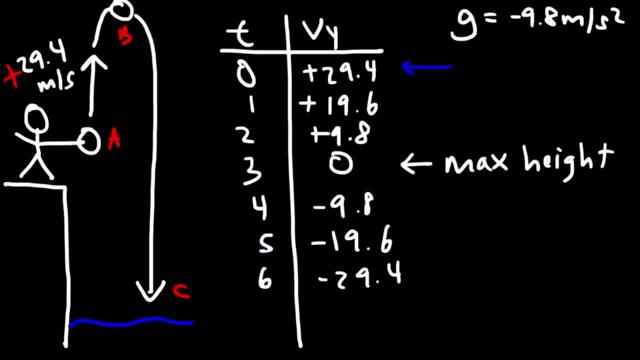 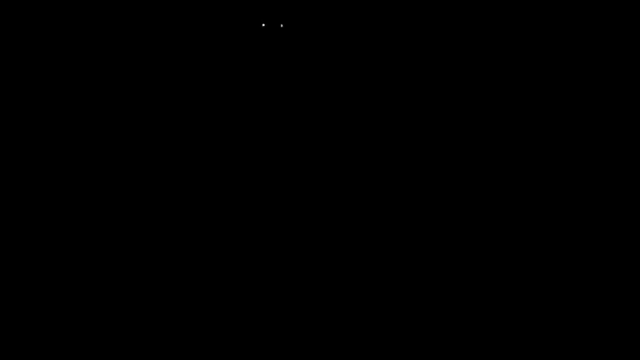 to the velocity values as time progresses. So anytime the acceleration of the velocity values is negative, the velocity is decreasing. As you can see, it started with a positive value and now it's becoming negative. Now, the next topic that you want to be familiar with is something called projectile motion. 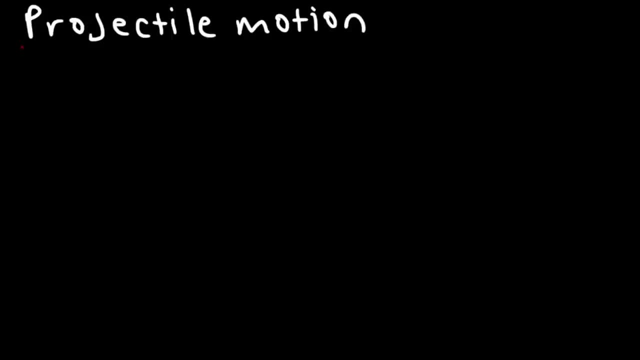 So what is a projectile? A projectile is basically an object that is moving under the influence of gravity. So in the last two examples, the ball that was released from rest and the ball that was thrown upward were behaving as projectiles because, once released, they were under the influence of 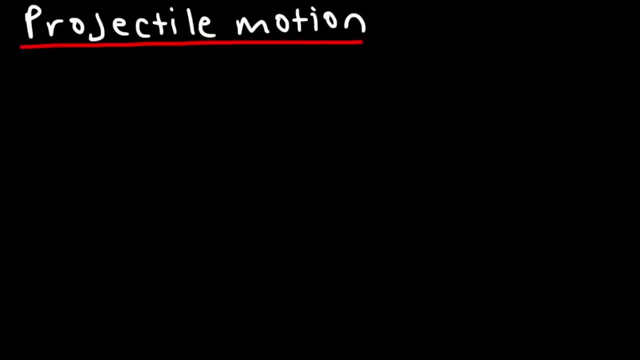 gravity, And in a typical physics course, when dealing with projectile motion, friction is usually ignored, And so we're not going to talk about it here. So far we've considered one-dimensional projectile motion, that is, in the y direction. The first case was a ball going. 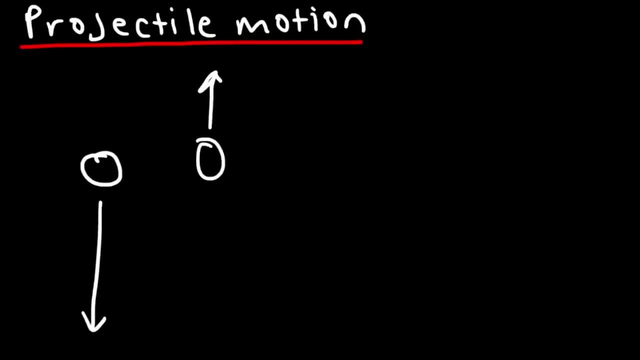 straight down. The second case was the ball going up and then down. So it's one-dimensional because it's only one direction, in this case the y direction. But let's talk about projectile motion in two dimensions, that is, in the x and in the y direction. So one example that you'll see is a ball. 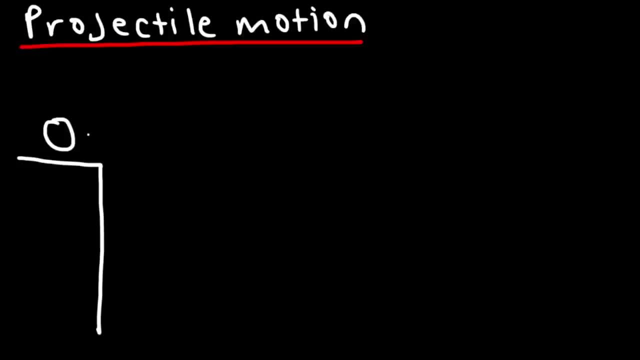 being kicked off a cliff or rolling off a cliff. Initially it's moving in the x direction and then it falls down like this, And so the path that the ball travels is known as the trajectory. Hopefully I said that right Trajectory. 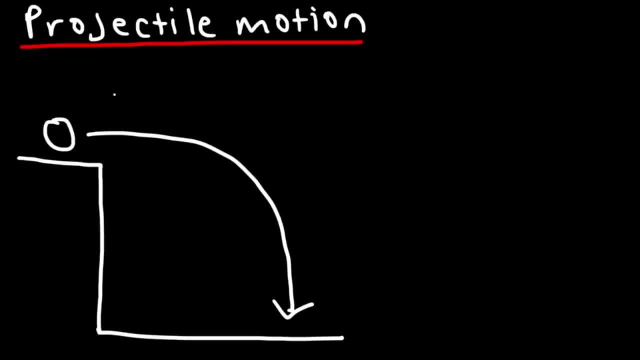 But now, let's say the ball was kicked off the cliff at a speed of, let's say, 5 meters per second. So what can you tell me about the vertical and horizontal components of the velocity of the ball at different times? So let's make a table between t, vx and vy. 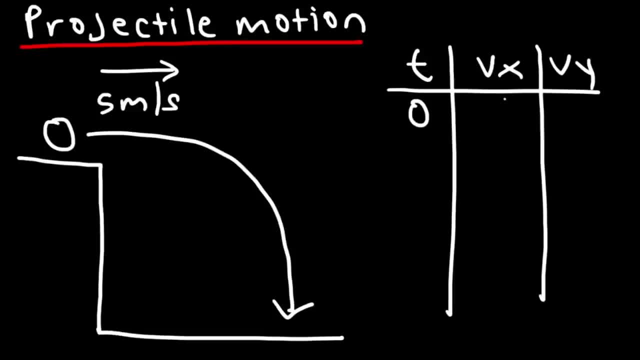 So initially, when t is 0,, vx is positive 5, because at that instant it's moving only in the horizontal direction. So if you look at the trajectory, this line is only going to the right. It's not going up or down, It's just going to the right. Now the vertical velocity is zero. 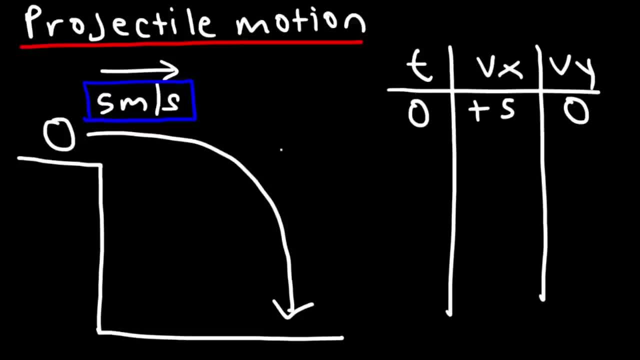 because it doesn't have any component in the y direction. Now, one second later, let's say, the ball is over here. So now the ball is moving in this direction. So the velocity can be broken up into its x component- So it's still moving to the right- And the y component- it's moving down. 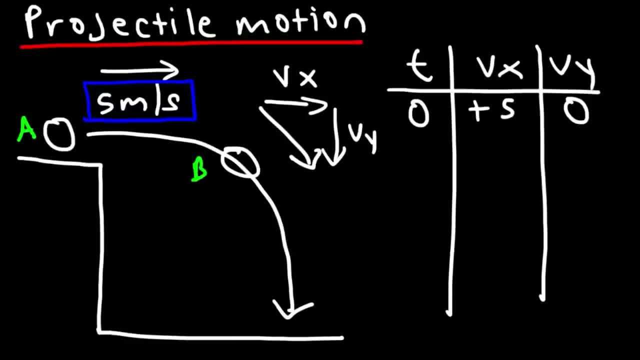 So let's call this point A and that point B. So at point B, because it's going in this direction, it has a vx value and a vy value. And let's say point B is one second later from point A. So point A, t is zero And at point B, t is one. So what is the velocity at point B? 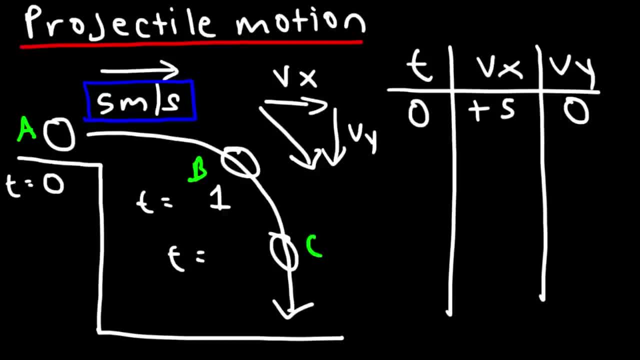 And what is the velocity at point A And what is the velocity at point B And what is the velocity at point C? let's say where t is two, two seconds, One second later, we know what vy is going to be, Due to gravitational acceleration. 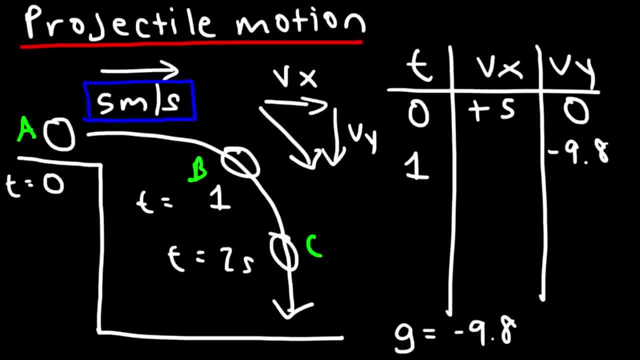 the vertical velocity will decrease by 9.8 every second. So two seconds later it will be negative 19.6.. Three seconds later, negative 29.4.. Now what about vx? Now it's important to understand that. g. 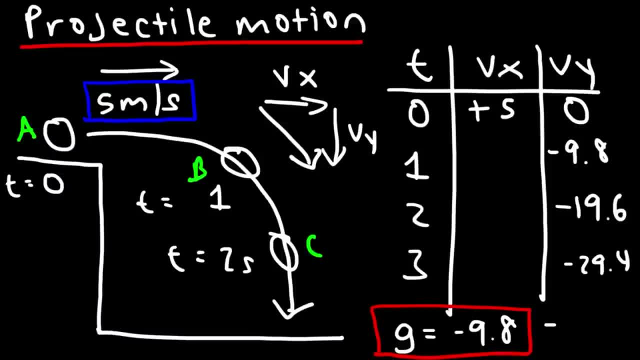 negative 9.8, is a vertical acceleration, not a horizontal acceleration. It's not a y, I mean it's not a x, but it's a y, So this number does not affect the vx. So when dealing with projectile motion, unless this ball has some rocket thrusters- 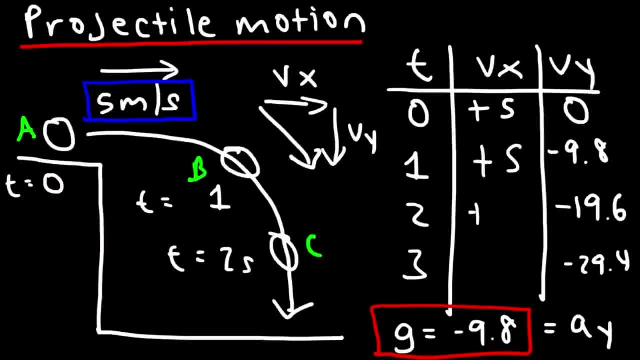 vx is constant, It doesn't change. So for projectile motion the acceleration in the horizontal direction is zero. So unless there's some kind of force that's propelling the ball to the right, that is, after it's been kicked ax is zero. 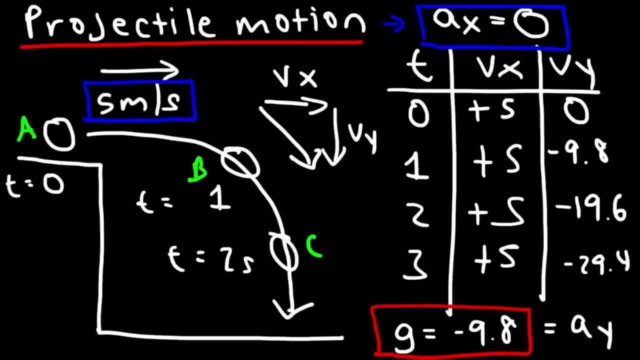 So it's important to keep that in mind. And if ax is zero, that means that vx does not change. If the acceleration is zero, the velocity is not changing. The velocity is constant. So to summarize what we've learned here, when dealing with projectile motion, it's important to understand. 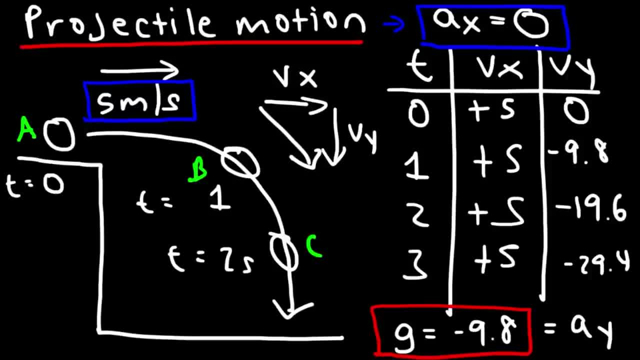 that the velocity in the x direction, vx, is constant. It doesn't change, unless the problem states that there's something accelerating it in a horizontal direction. If there's no specific statement, as such, ax is zero and vx is constant. But for any projectile motion problem, vy changes. 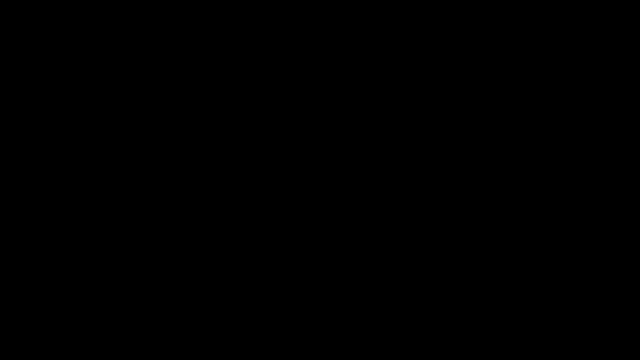 vy is going to change by 9.8 every second. Here is another projectile motion situation. Let me start at the bottom. So let's say we have a ball and the ball is kicked off the ground at an angle. It goes up and then it goes down. Now, typically, 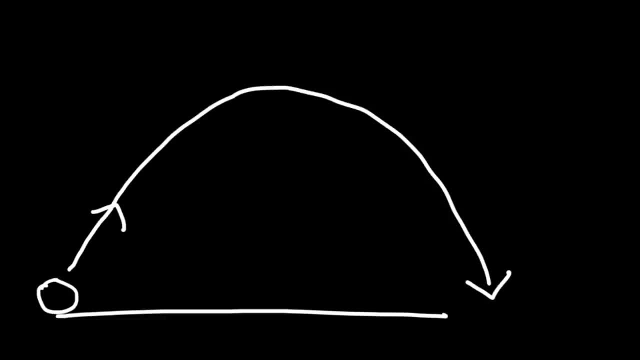 you might be, given the velocity at which it's kicked. Let's say it's going up at a speed of 40 kilometers per second, And let's say it's at an angle of 30. So you have v, which is 40,, and you 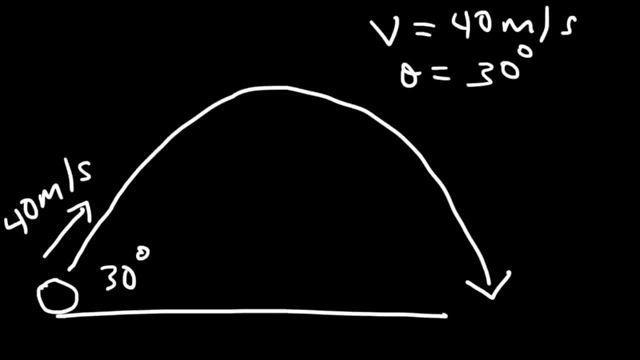 have the angle theta, which is 30 degrees. Now what you need to do is find vx and vy. vx is basically v cosine theta, And this is the initial value. vy is v sine theta. Now for this problem. I'm going to 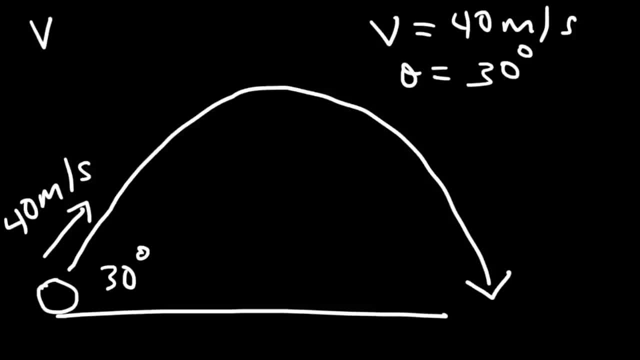 give you vx and vy, And I'm going to give you v, cosine, theta. Now for this problem, I'm going to give you Vy, So we're going to choose some different values. but in a typical problem, when you're given V and theta, you can find Vx and Vy using those formulas. But let's say that you discover. 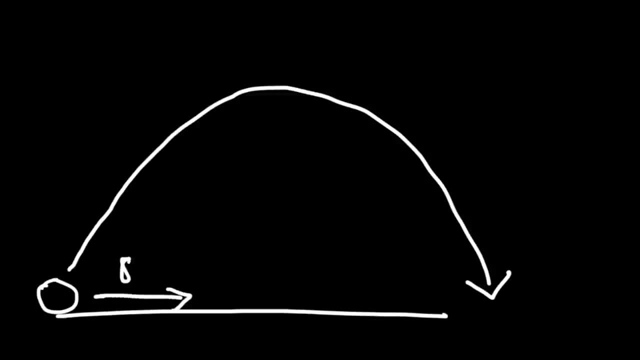 initially, Vx is- let's use a nice number- 8 meters per second, And Vy, we're going to say, is 29.4 meters per second, So that's at a time value of zero. What's going to happen one second later? 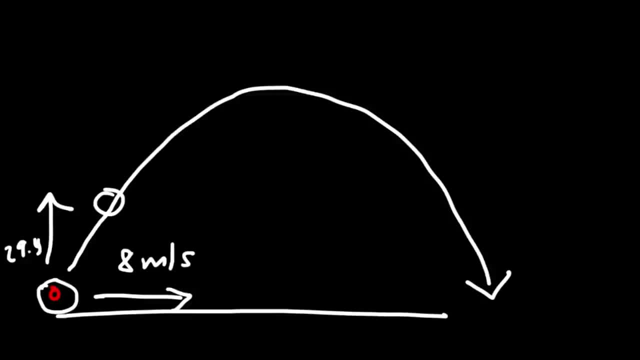 So, one second later, what's going to happen to Vx and Vy? Now it's important to understand that Vx will not change, for projectile motion Gravity does not affect Vx, it affects Vy. So one second later, Vx will change. 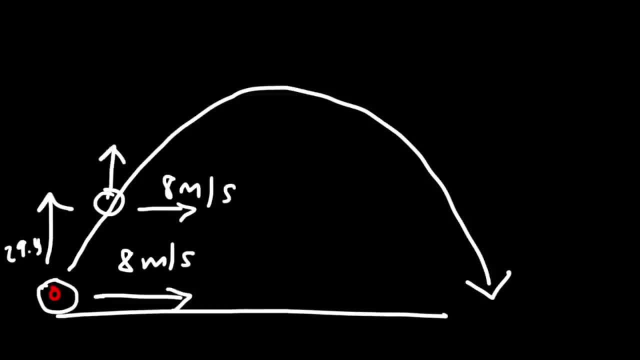 still be 8 meters per second. Vy is going to decrease by 9.8 meters per second. every second Gravitational acceleration affects Vy, but not Vx, So this is going to be 19.6. one second later. Now, two seconds later, Vx will still be the same, and that's 8 meters per second. 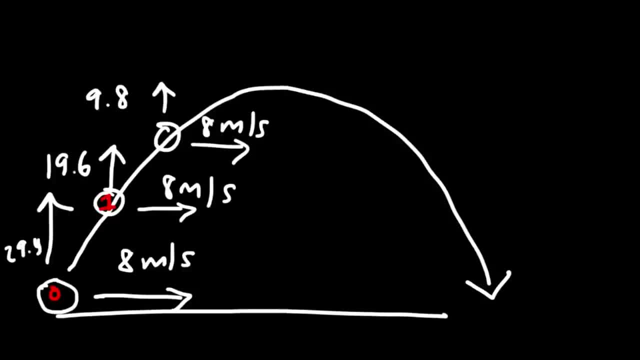 Vy is now 9.8.. Three seconds later it's at the top, at the maximum height, at the highest point. Vy is zero, so it's not going up anymore, but it's still moving to the right. so it's still moving at eight meters per second to the right. so that's Vx. 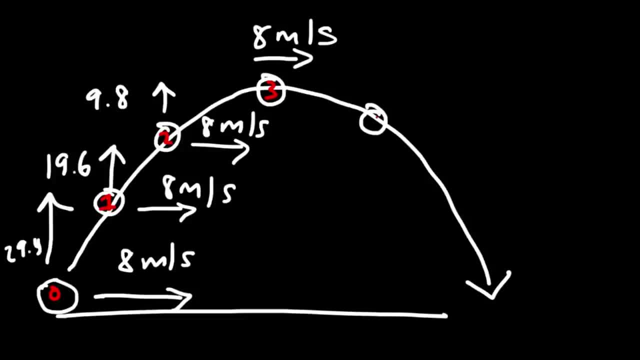 Now, four seconds later, what do you think is going to happen? Well, Vx is still the same. it's still 8 meters per second, but now it's going down. so Vy is negative 9.8.. And then, five seconds later, Vx is still the same. 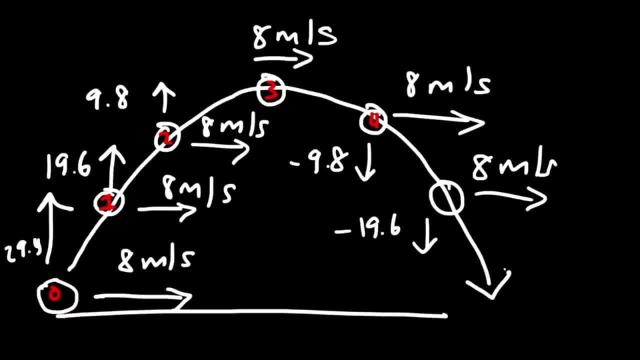 but Vy is now negative 19.6.. And six seconds later Vy is going to be negative 29.4.. So notice that Vx is still the same. The speed is the same when the height is the same if the trajectory is symmetrical. 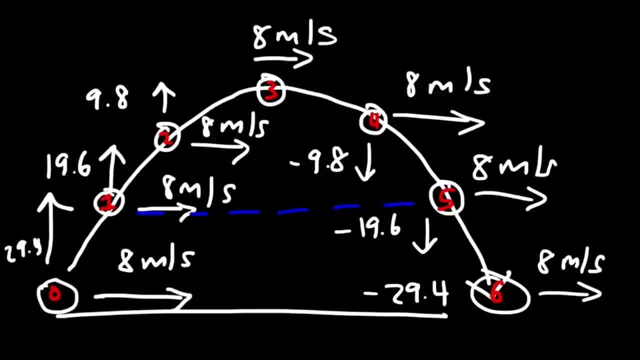 In this case the left side looks exactly the same as the right side, so there's symmetry for this type of shape. So at a certain height Vy has the same magnitude, but the opposite sign This is positive 19.6, and that's a negative 19.6.. So the velocities just have opposite signs. 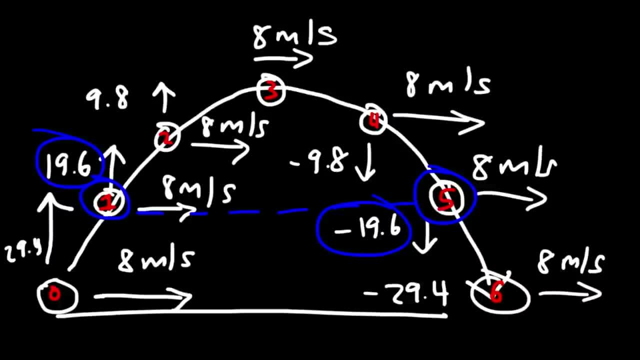 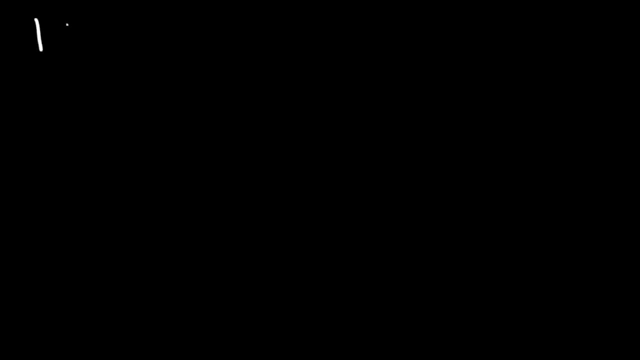 But speed in either case is still positive 19.6.. So the speed is the same when the height is the same. But Vx doesn't change in the typical projectile motion problem. Only Vy changes based on the gravitational acceleration. Now let's talk about Newton's three laws. So let's go over the first law. The basic idea behind Newton's first law is that Newton's first law is the same as the first law. 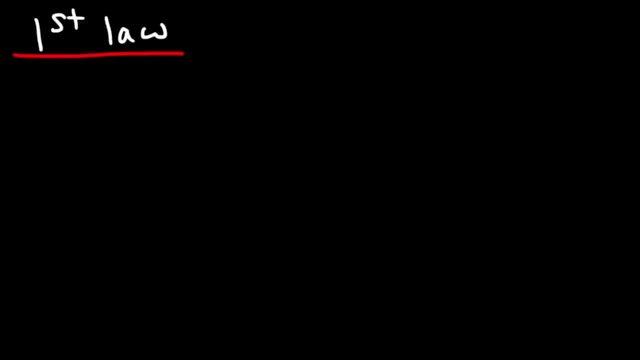 The basic idea behind Newton's first law is that Newton's first law is the same as the first law. The basic idea about Newton's first law of motion is that the object at rest will remain at rest unless acted on by a force And the object in motion will continue in motion unless acted on by a force. 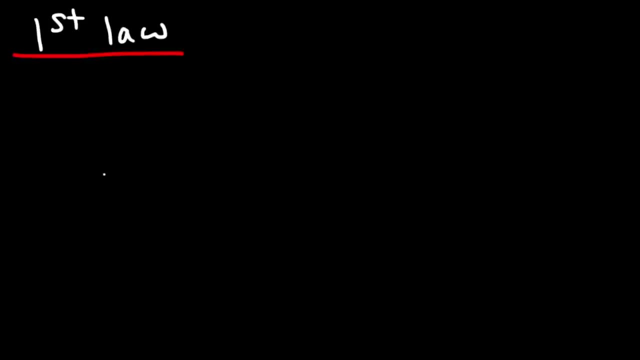 Therefore, an object in motion will remain on by a force. So let's say, if we have a box and its at rest, it is not moving. The only way we can get this box to move is by applying a force. A force is a. 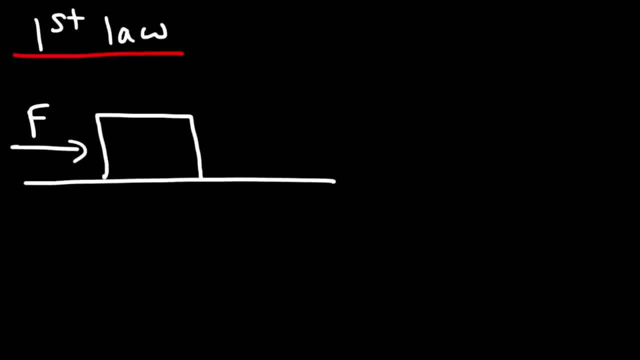 is a push or pull action. so in this case the force is pushing the box towards the right. we can also get the box to move towards the right if we take a rope and pull the rope towards the right. so here this is a push action, and towards the. 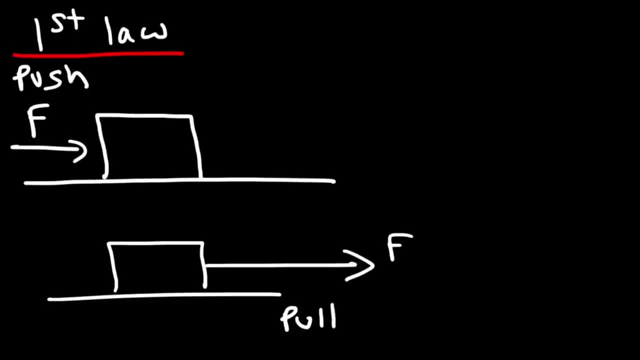 right, it's a pull action, and the way to pull something is by means of a rope. whenever you have a force acting on a rope, it's known as a tension force. so whenever you hear the word tension, it's basically a force acting through a rope. so unless we apply a force, the box at rest will continue to remain at rest now. 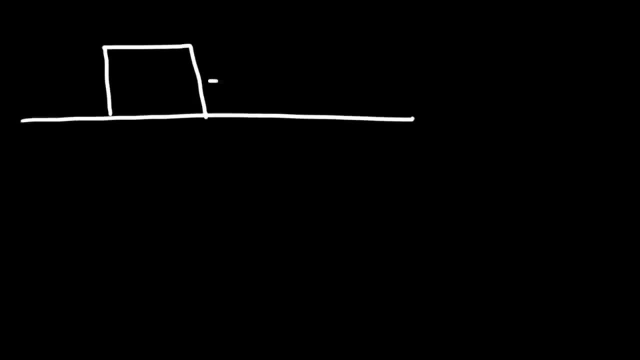 let's say we have a box and this box is moving towards the right, and this box is moving towards the left and this box is moving to the right, so it's sliding across the surface. the only way to stop the box from moving in this direction is to apply a force in the opposite. 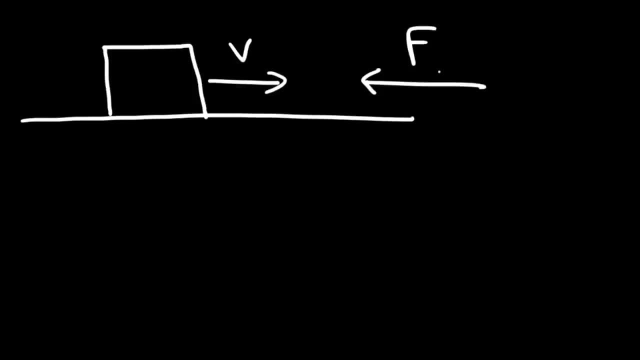 direction, and friction will do that too. so if you try to slide a box across a rough surface, you know the box is going to come to a stop, because friction will oppose the box moving. friction always opposes motion. it tends to slow things down. and so thus we have Newton's first law: an object in motion will continue in motion unless 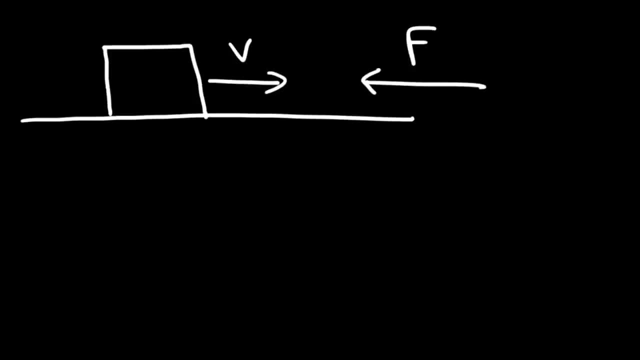 acted on by force. so if there was no friction, this box will continue to slide forever. but because friction is present and it's opposite to the direction of the velocity of the box, it's going to slow it down and bring it to rest. so if that force wasn't present, it will keep moving. so if you think of objects, 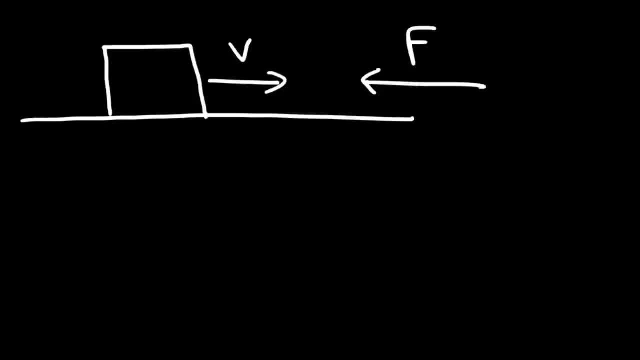 moving in outer space where there's almost no friction, those objects tend to basically move forever. so if you think of the earth as it revolves around the Sun, the earth moves in a vacuum of space, is basically almost no air in space and so that there's hardly any friction does it can move forever around the Sun. 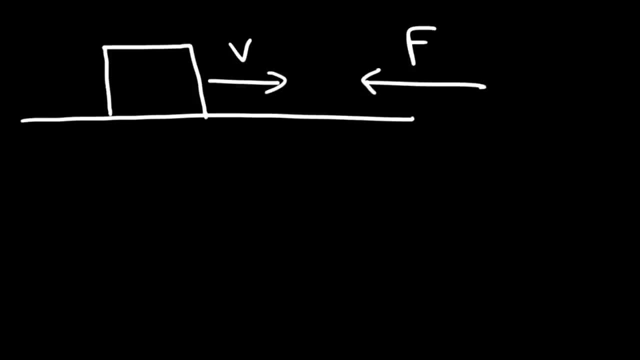 without friction, any or hardly any assistance. a good way to illustrate this is: imagine if we take an object and let's say, like a puck if you're playing air hockey, and if we slide it across ice- because it's not much friction between this object and ice, because ice has a very smooth surface- this object will travel for a 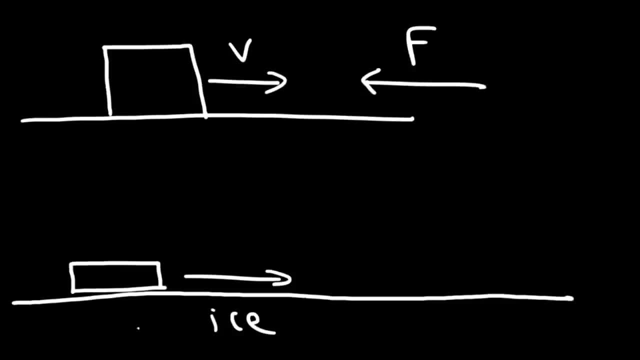 very long time because there's not much friction between the ice and this object, whereas, let's say, if you have the same object across a rough surface, this object will not slide very far. it's going to come to a stop quickly because it's more friction, and so if you 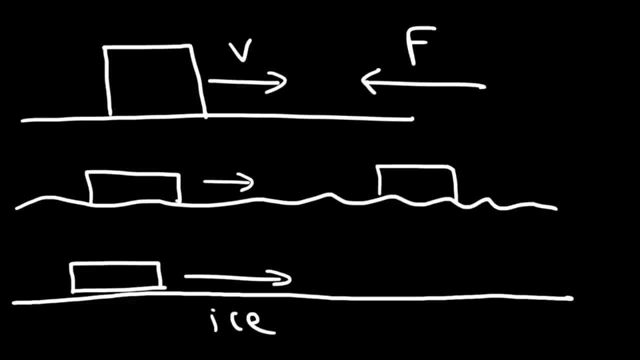 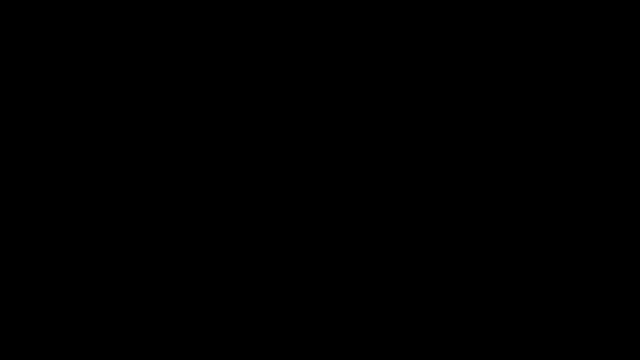 can reduce friction, the object will travel for a very long time. if you can completely eliminate friction, then by Newton's first law of motion, it should continue forever. so an object in motion will continue emotion, unless acted on by force. now let's talk about Newton's second law and the best way to summarize Newton's.